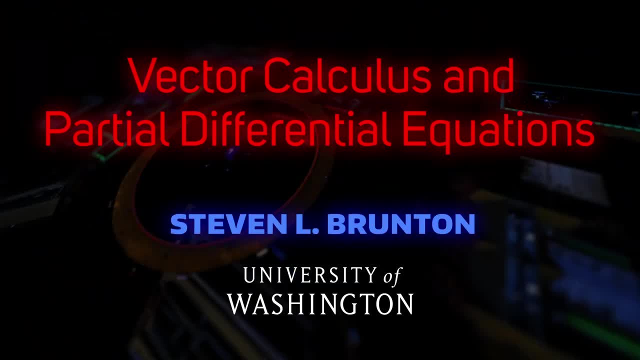 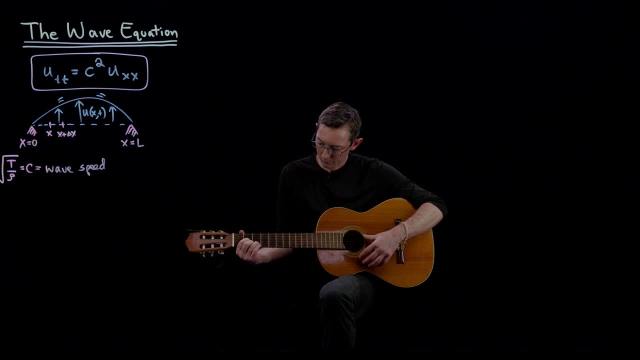 Welcome back. Okay, in the last lecture we derived the wave equation for a vibrating guitar string from scratch, from f equals ma, physics, literally just, you know, conservation of momentum of a little infinitesimal section of guitar string vibrating up and down. you know, being forced by 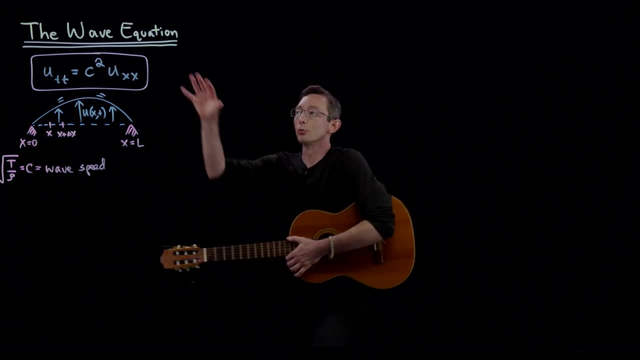 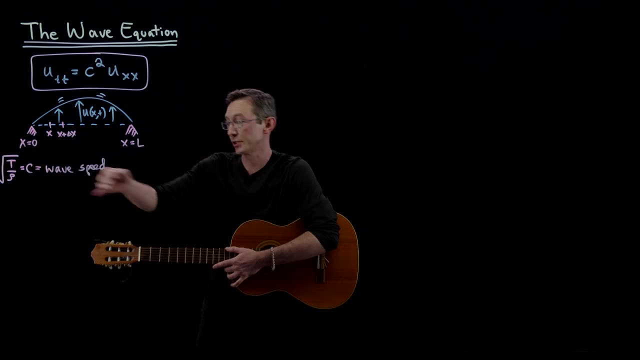 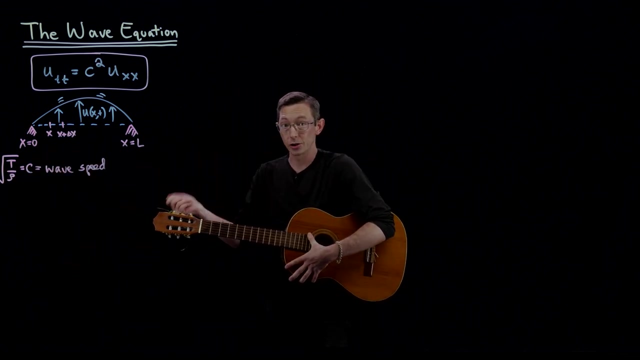 its own tension, essentially the tension in the string. So we derived this equation from scratch. where the wave speed c is related to the material properties of the guitar string, C is literally the square root of the tension divided by the linear density. So increasing the tension increases the wave speed, which makes higher pitch sounds Decreasing. 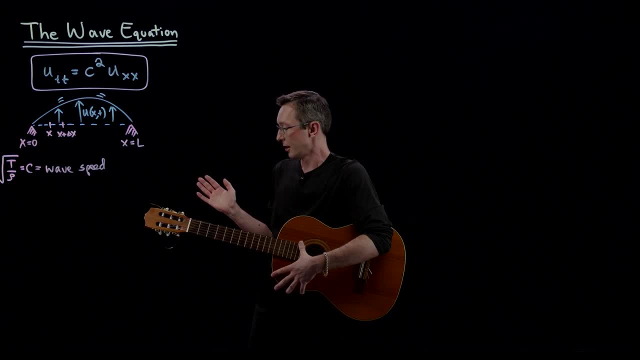 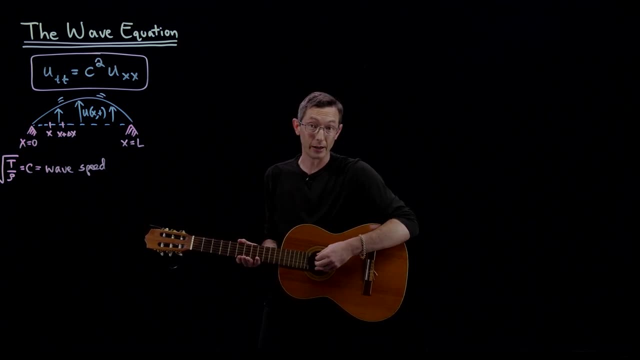 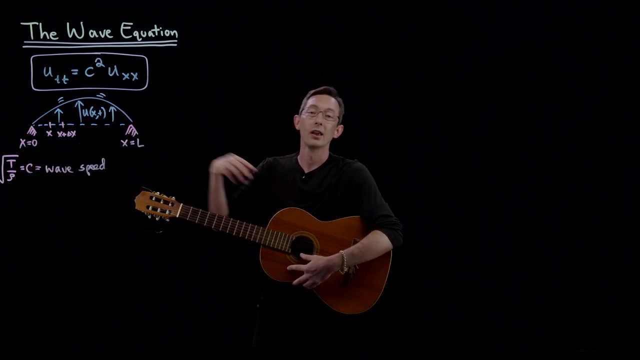 the tension makes it lower pitched. I massively detuned my guitar last time but it's back to in tune And the linear density. a thicker string, a thicker, heavier string like the low e, will have a lower wave speed because it has a higher row than a thinner, lighter, high e string. 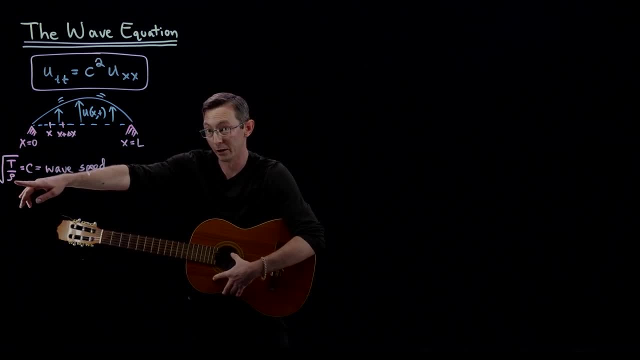 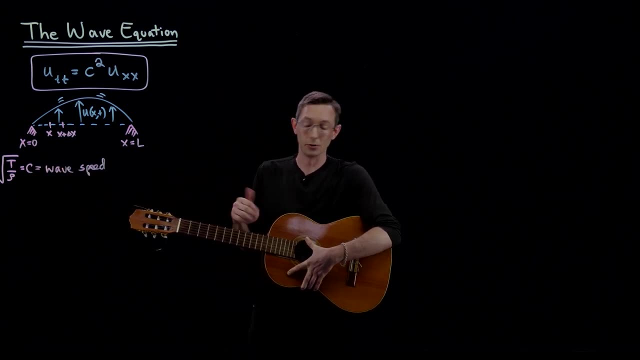 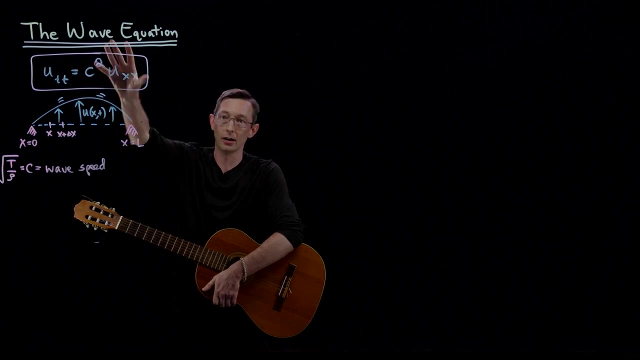 Right. So this one, the low one, has a bigger row- smaller c. The lighter one has a smaller row, higher c, And that translates to either a lower-pitched sound or a higher-pitched sound. So what we're going to do today is from this wave equation. we're now going to solve this. 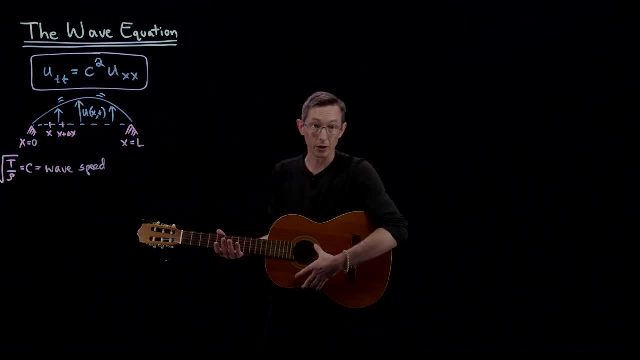 for some specific boundary conditions, literally for this guitar boundary condition where it's pinned kind of here and here at the bridge and at the neck, And then we're going to analyze what happens, you know, to this wave equation. What happens, what are the solutions of this wave equation? 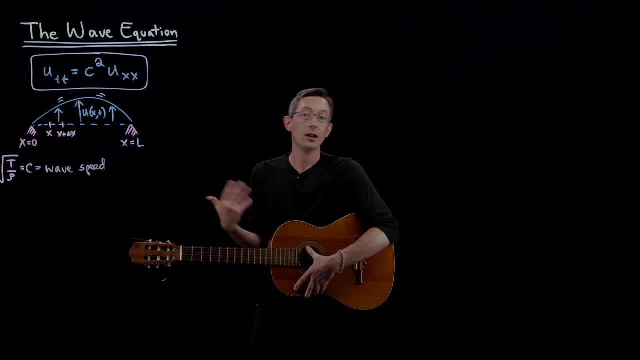 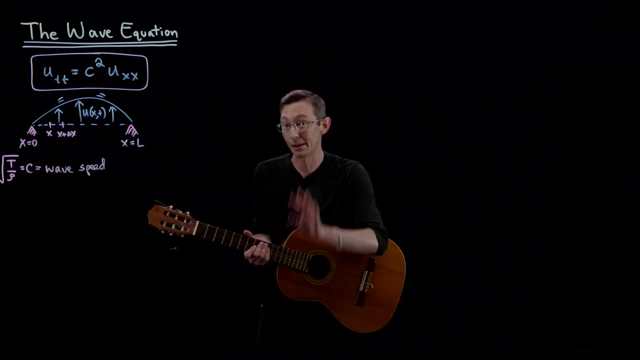 And how does that translate into intuitive things we know, you know from music, from sound, from things like that. Okay, So that's all coming up and we're going to solve this using separation of variables- one of the most important solution. techniques for partial differential. 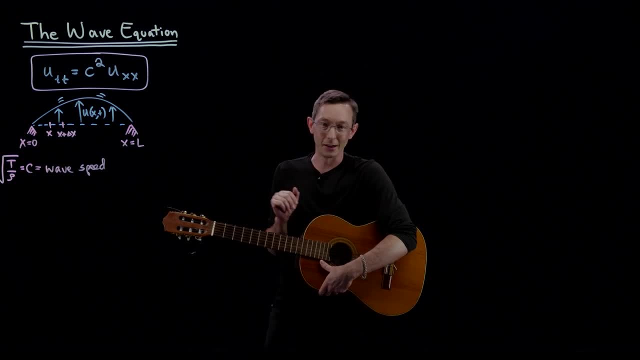 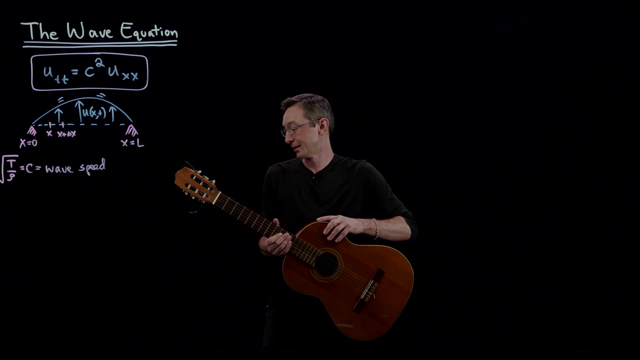 equations. I want to point out just: I hope you appreciate. I hiked my guitar up three miles from home to film today, So I hope you appreciate the dedication. I hope you appreciate the dedication. I thought about just playing air guitar, but I figured this would be a lot more interesting. 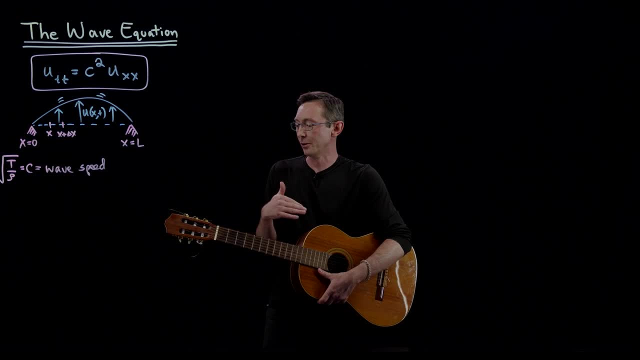 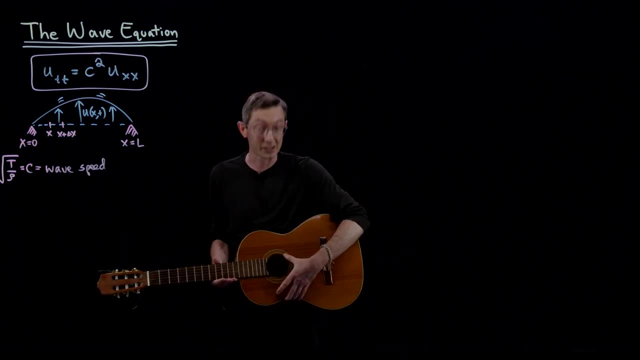 Just a preface at the very beginning. you know I am a complete amateur novice. I know zero music theory. My wife likes to joke that you know, all I know is string theory for the wave equation and the string. I don't really know any music theory But I do think that this is a really intuitive 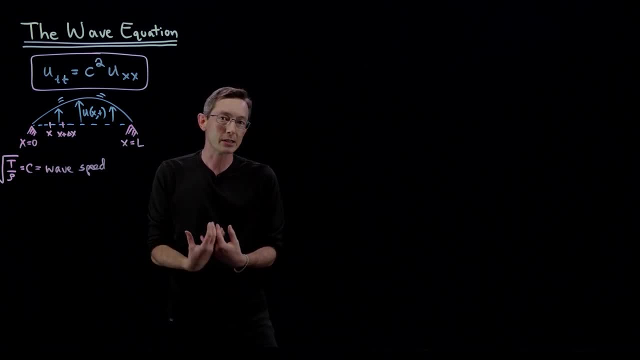 kind of example, because music, much like mathematics I think, resonates with music. It resonates very much with the kind of logical part of our brain but we also know when it feels right. And so that meeting place of kind of thought and feeling I think is very much shared. 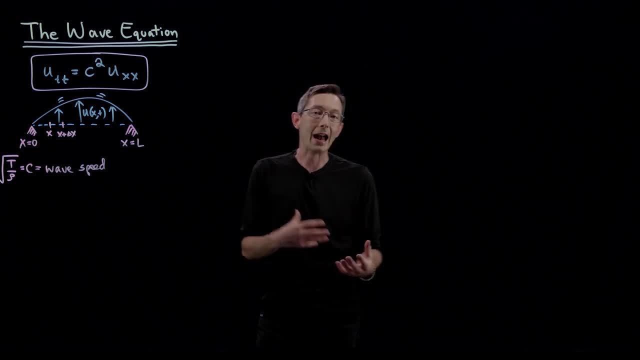 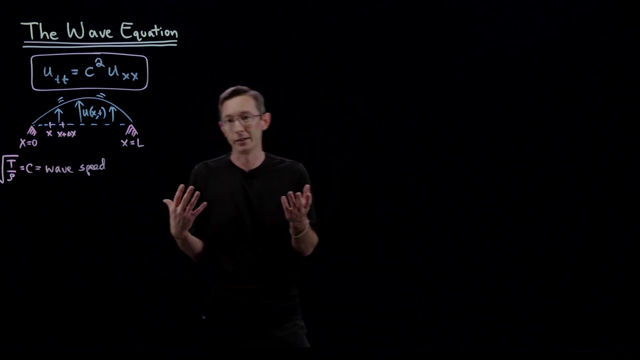 between mathematics and music And in fact there are deep, deep connections between music and mathematics that people have been exploring and uncovering for hundreds of years, for centuries, if not millennia. So even if you go back, this is a little bit of just a history digression, but I think it's interesting. 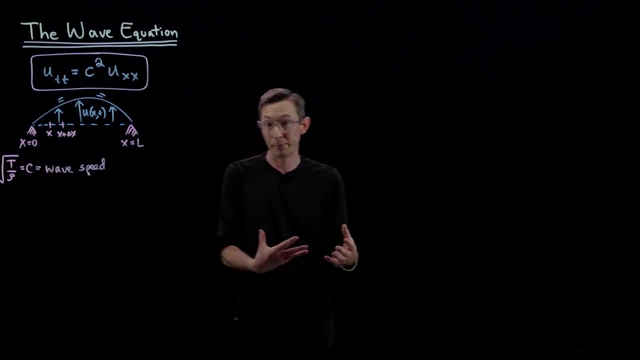 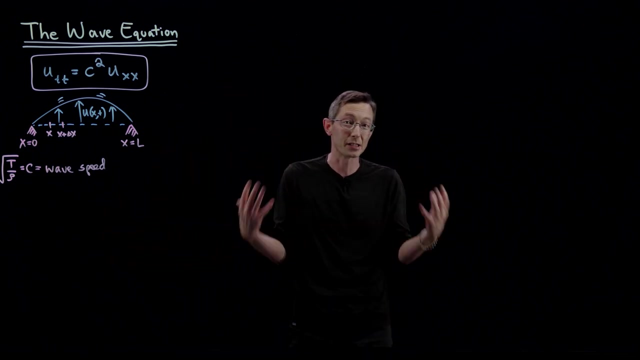 If you go back to you know, Tycho Bray and Kepler before Galileo, before Newton, before we knew about F equals MA and before we had, you know, proven that the sun was the center of the solar system, when things were still speculative and people didn't understand why the planets 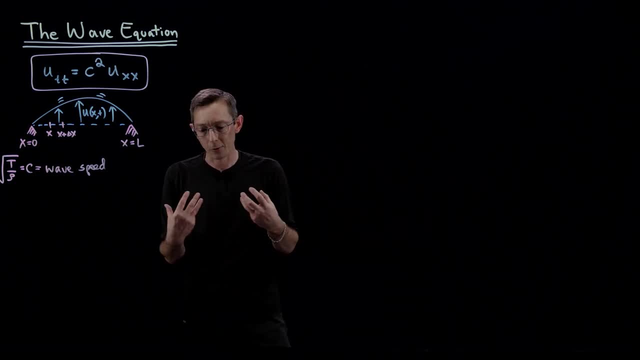 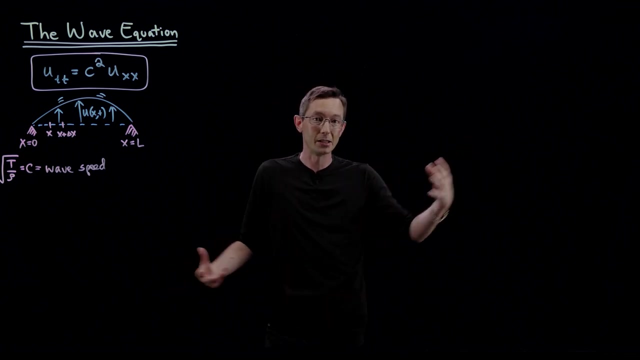 behaved the way that they did. there was a theory- and Kepler held on very strongly to this theory- that there were harmonic patterns in the motion of the planets and the motion of the stars, just like musical patterns and layers, you know that define musical composition. They believed. 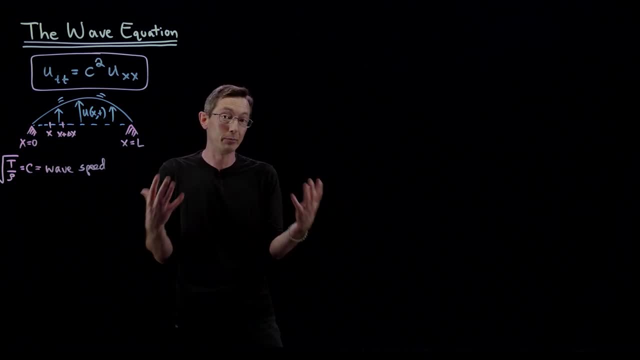 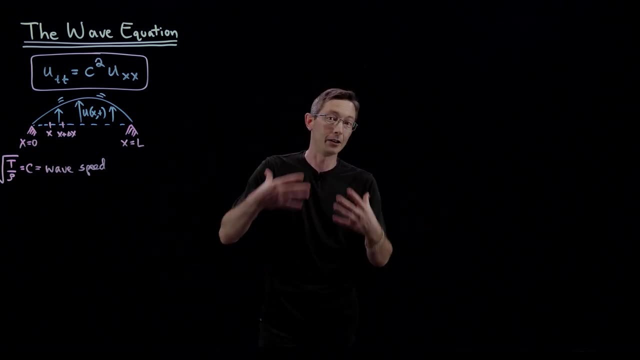 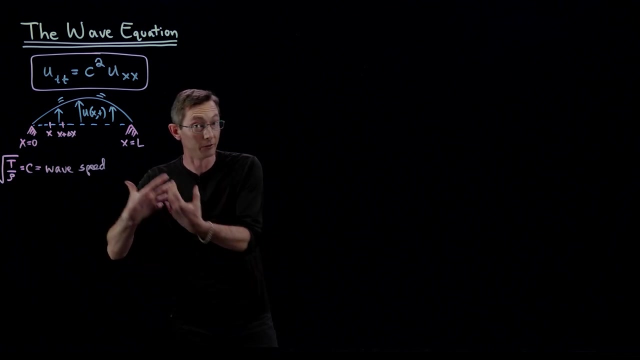 that there were these patterns in the stars and the heavens and the planets, and that that musical composition was perhaps divine and definitely had an impact in our daily lives. right, This is astrology, you know from the olden days. It always had this flavor of you know. 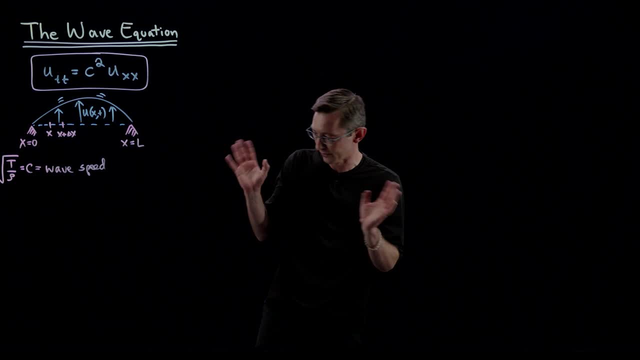 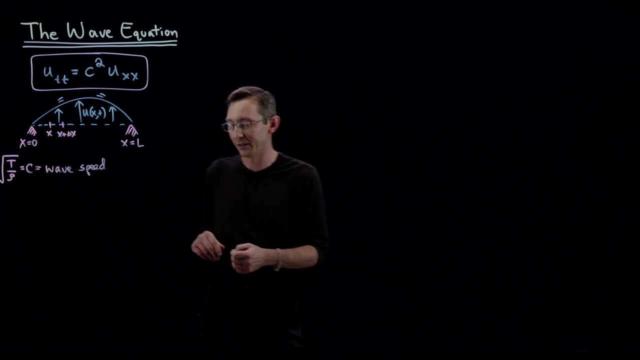 one part mathematics and one part music. Just fascinating, I think, Oh and yeah. in lugging my guitar to work today, I was thinking back. a friend of mine taught me a new word called busking. So busking is when you bring your guitar or musical instrument and you play in. 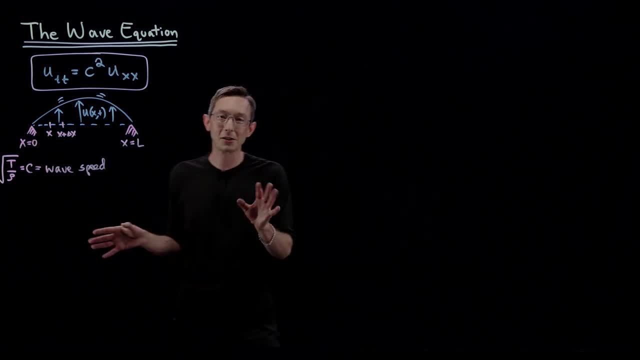 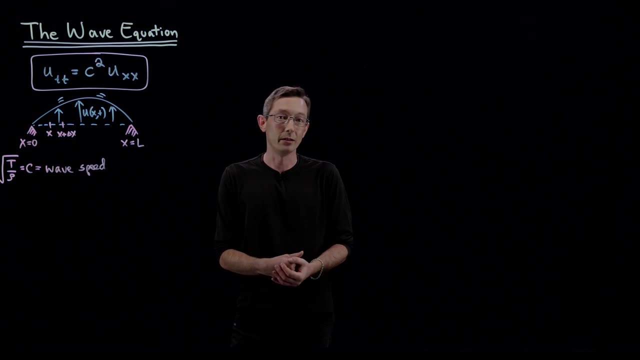 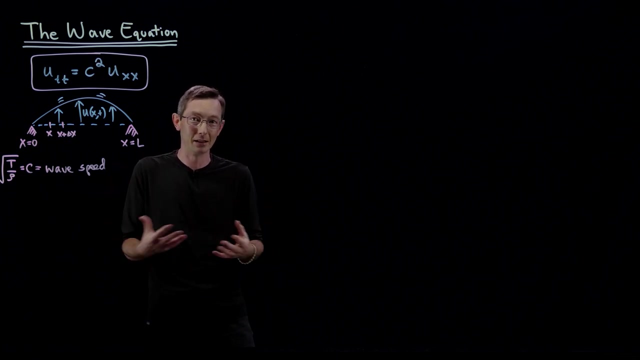 public, in a public space, and I think it's a super fun busking. It comes from the Spanish word buscar, which means to seek, you know, seek out something, And so we are, all you know, in some sense busking and buskers, because we're. 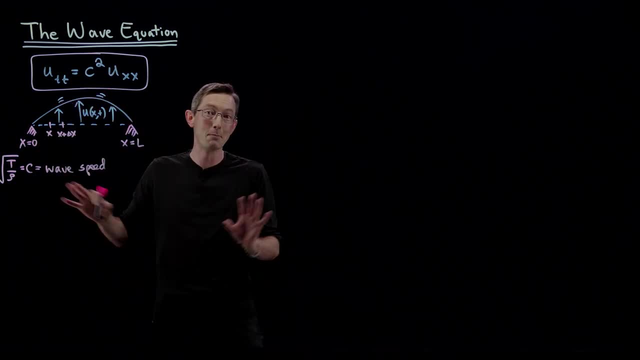 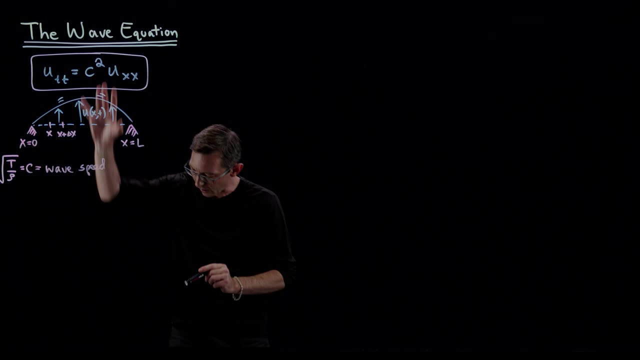 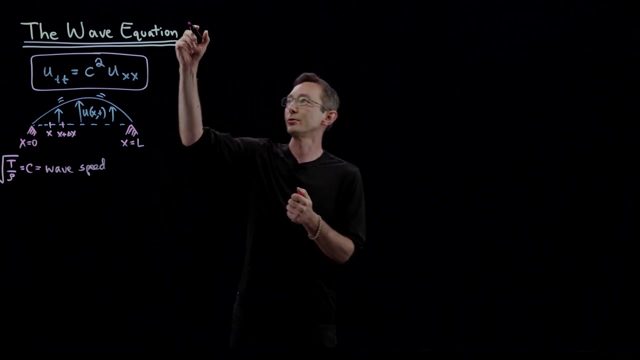 all seeking knowledge. This is a very, very meta. you know, two steps removed, online YouTube version of busking, I suppose. Okay, good, So I'm going to jump right into this. We're going to solve this equation using separation of variables. Maybe I'll just write it here: Separation of variables. 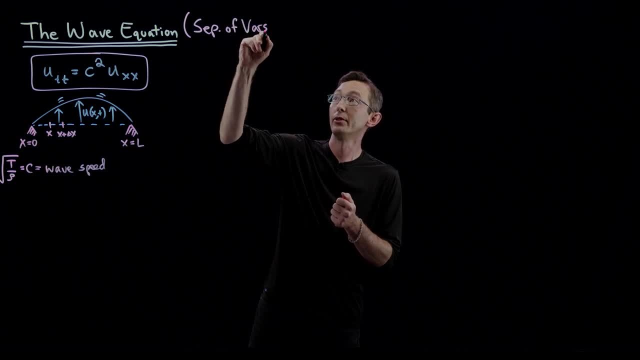 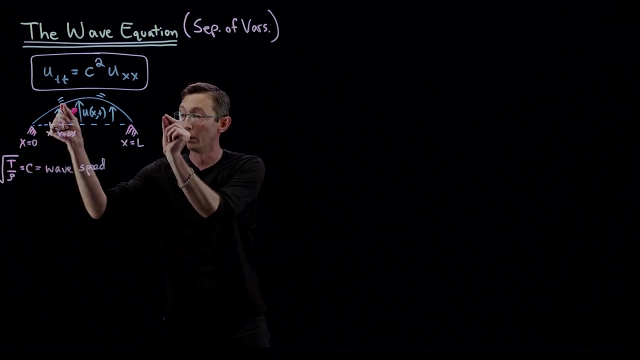 which we've already solved. We've already seen before, when we solved Laplace's equation for the heat distribution in a rectangular metal plate. Here we're going to solve for kind of you know, the vibration, the motion of the string where it's pinned in two locations, at x equals zero and x equals l. L is the length of. 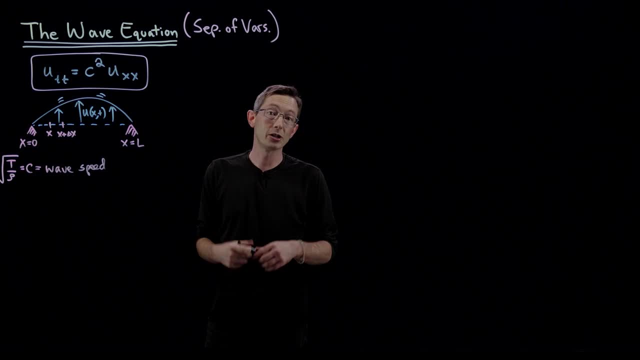 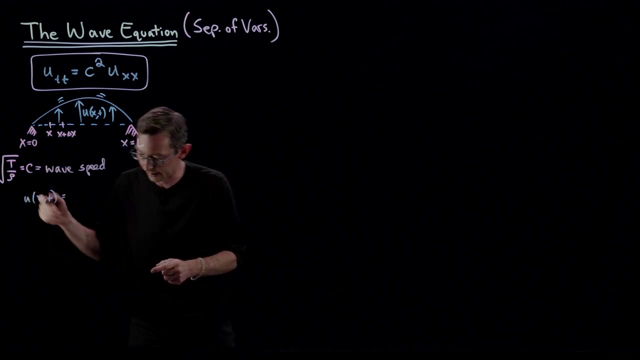 my string. And so, again, for a partial differential equation to be well defined, we need to define its boundary conditions and its initial condition. So I'm going to do that, I'm going to do that here. I'm going to say, just to be very, very clear: u of x and t is the height. 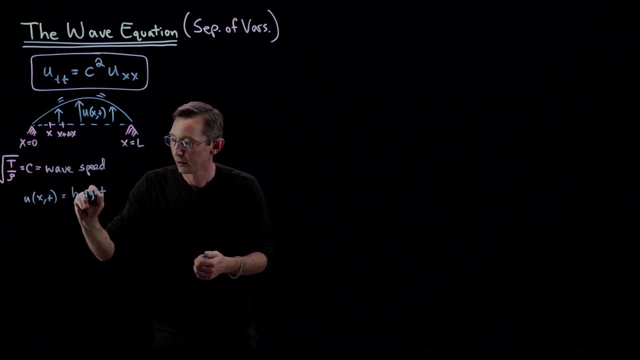 of the string, the height or the displacement of that string, the displacement of the string, And it's going to be a function of x, the position along the string, and in time, It's going to be oscillating in space and in time And our boundary conditions, our boundary conditions. 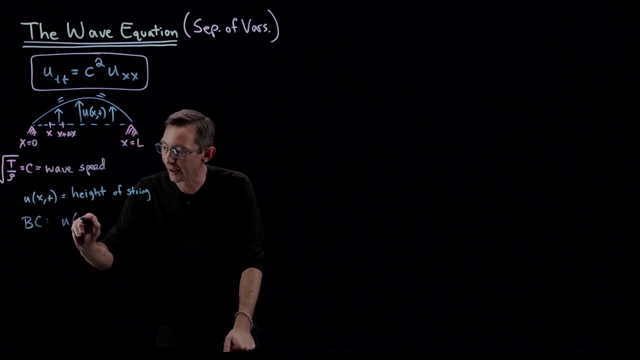 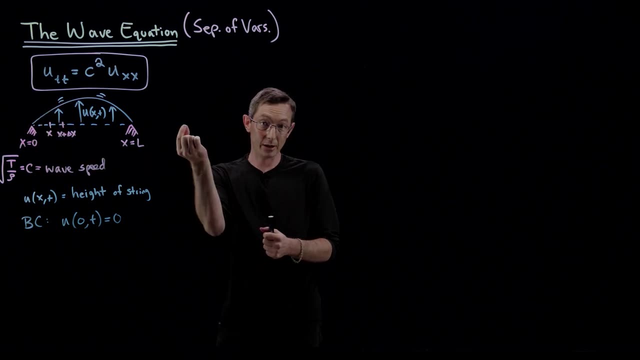 are essentially u at x equals zero for all. of time is going to equal zero. So we've essentially pinned the string in one position, up at the neck, And that is going to be a zero displacement for all time. This is at the neck And similarly at the bridge at the other end of the string. 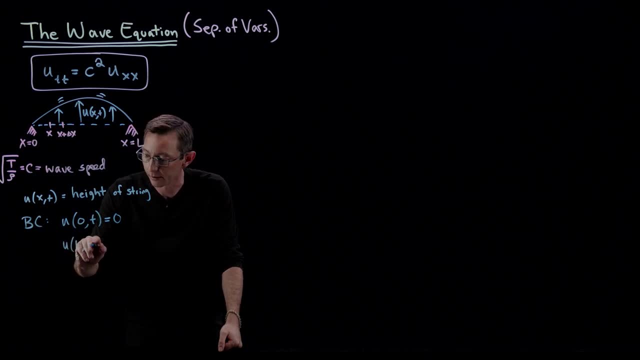 u of- sorry it's so squeaky- is also equal to zero. So at length l for all time. it's also pinned in that location. But it can kind of do whatever it wants in the middle. okay, So I can, you know, deflect the string. You know I can pull the string with. 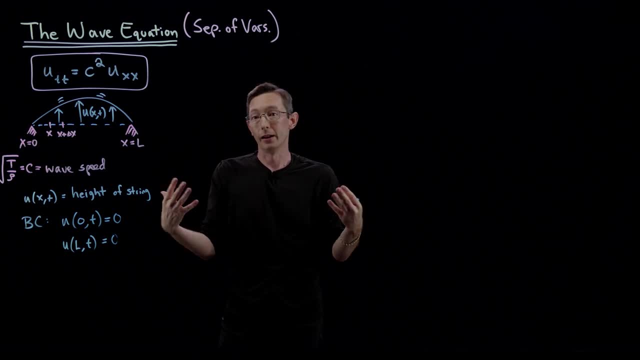 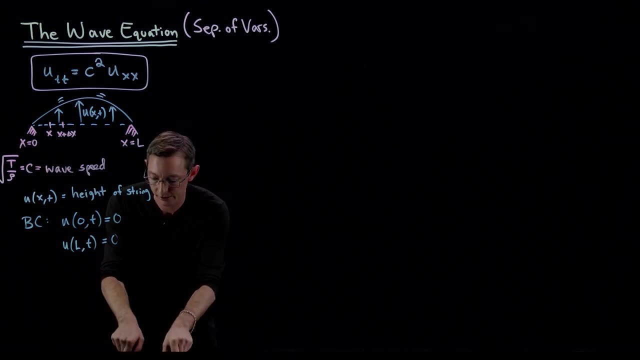 my finger and make it a little shallow triangle. That's totally fine, as long as it stays pinned at both of the boundaries. And then the last thing I need is my initial condition. Maybe I'll switch colors so it's not so squeaky. Oh, still squeaky. My initial condition is going to be u at x at. 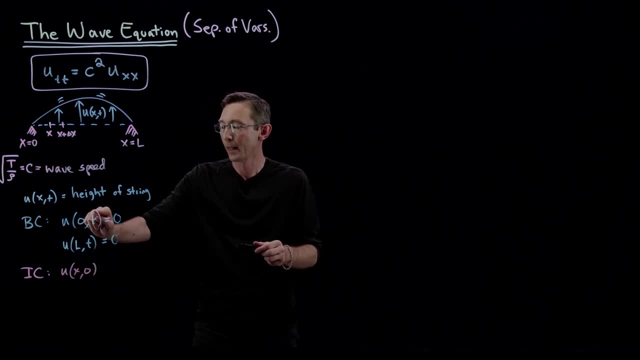 times zero. So I'm going to do that, And then I'm going to do that, And then I'm going to do that. So now, remember, my boundary conditions are for all time. at spatial boundaries, My initial condition is, at a given time, at my initial time, t zero at all of the positions x. I'm just going. 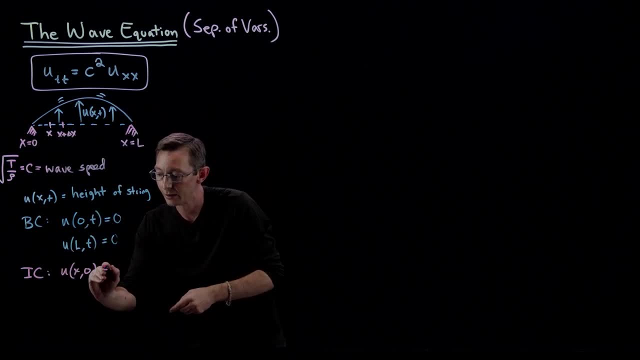 to define the displacement at time zero to be some function of x. And this function of x could be: you know that I take my guitar string and I, you know, essentially pull up on the guitar string in one place and then I let it go. That could be my f of x. is that it's. 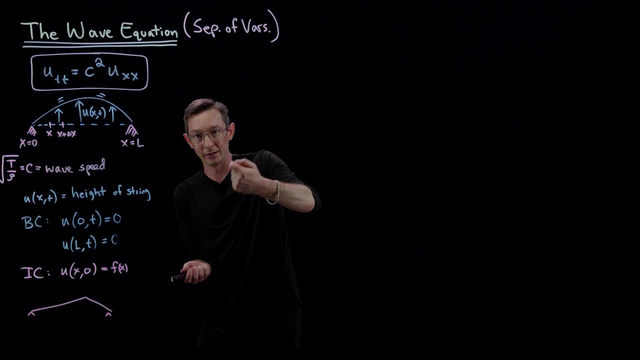 this little triangle from me pulling up, you know, and about to, with my pick or with my finger. So I have boundary conditions and initial conditions which make this a well-posed partial differential equation. It's a linear partial differential equation. 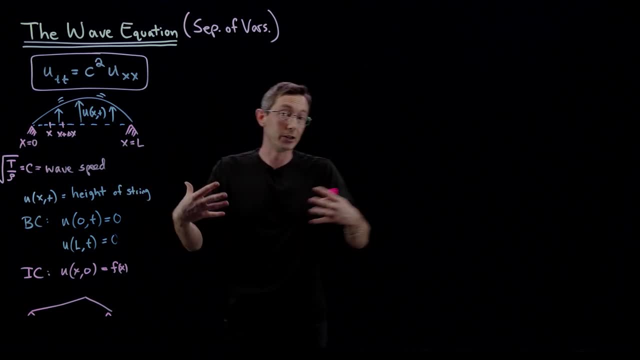 which means that superposition holds. It means that if I have, you know, multiple solutions and I add them up, if I have multiple solutions that satisfy my boundary condition and I add them up, then they're still going to be a solution of my partial differential equation. 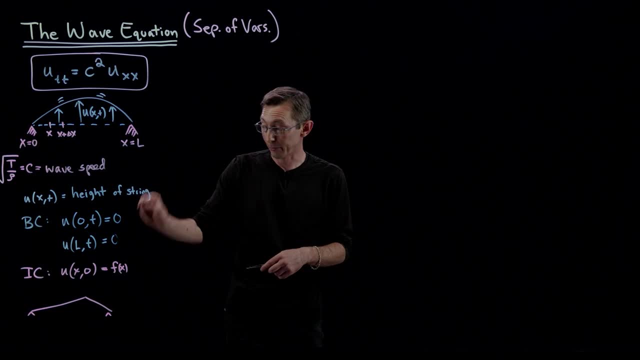 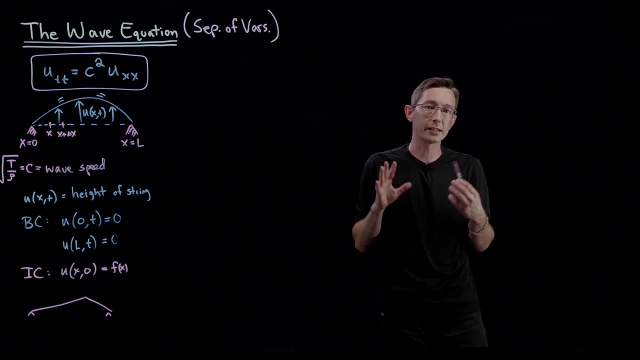 That's nice, And we're going to solve this using separation of variables, just like we did before. So I'm going to jump in. So our separation of variables assumption: the basic, basic assumption here is that u of x and t- my function of space and time- is separate. 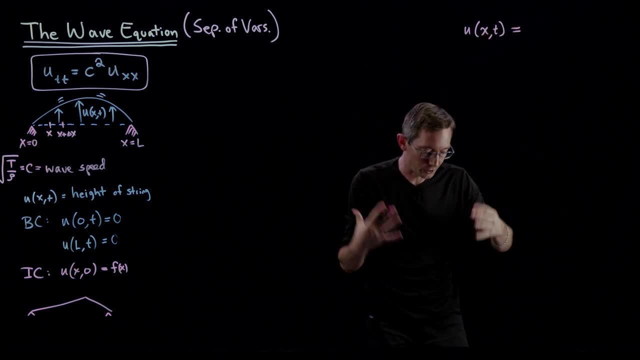 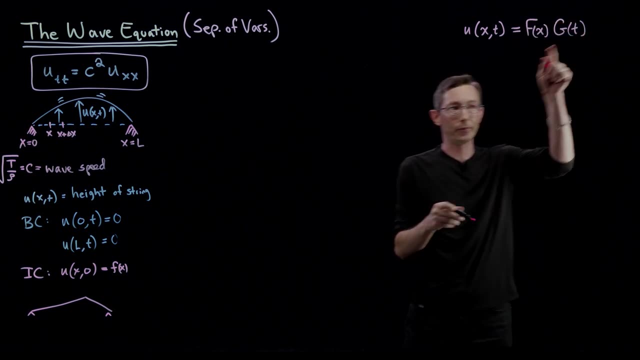 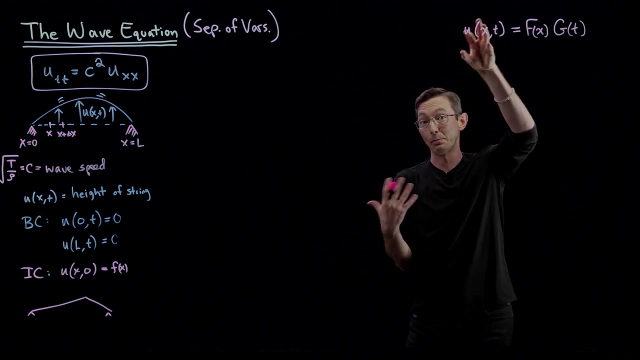 separable, which means that I can write this as a product of a function just of x, f of x times a function g. that's just a function of time. So this is the basic, basic assumption of separation of variables: is that I can say that my solution, which varies in space and time, 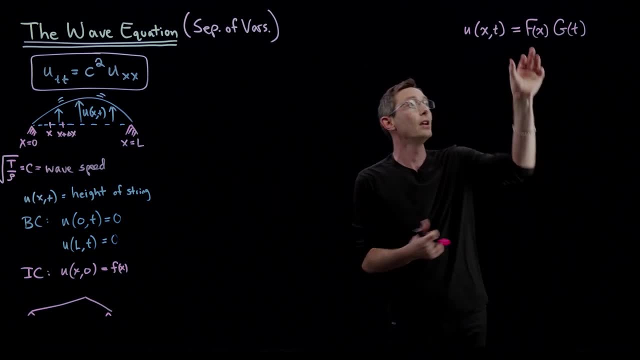 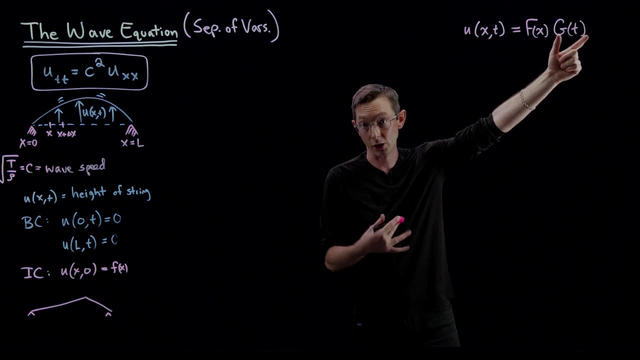 remember that that guitar string is vibrating in space and in time. but I'm going to assume- this is an assumption- that it can be written as a product of a function just of space times, a function just of time, And when we plug this into our PDE and go through all of the steps, we're going to see if that 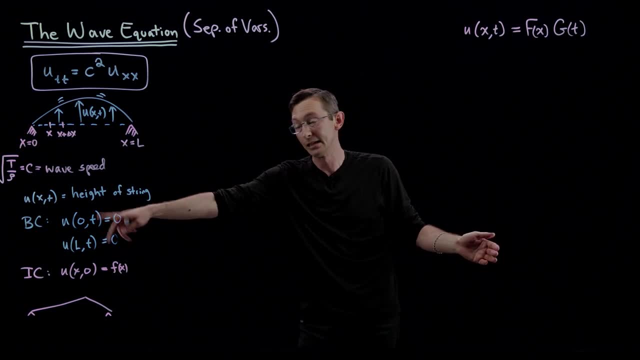 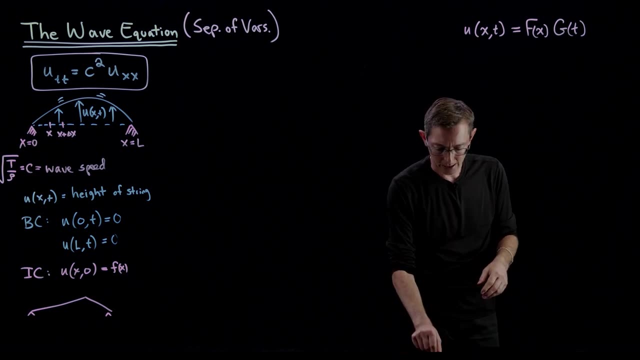 assumption holds and if we can get a solution that satisfies these boundary conditions and initial conditions, Good. So that's what we're going to do, And maybe I will just start writing out what the derivatives are. I think that's a good place to start. We're going to plug it into. 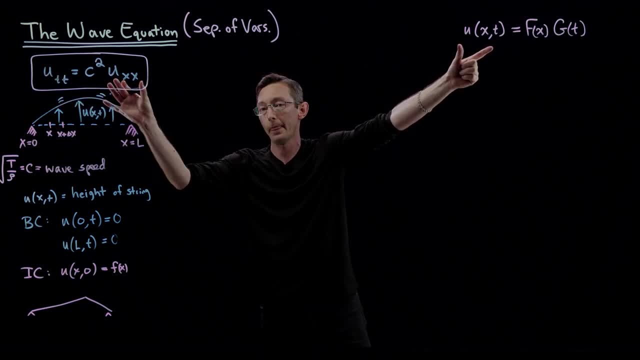 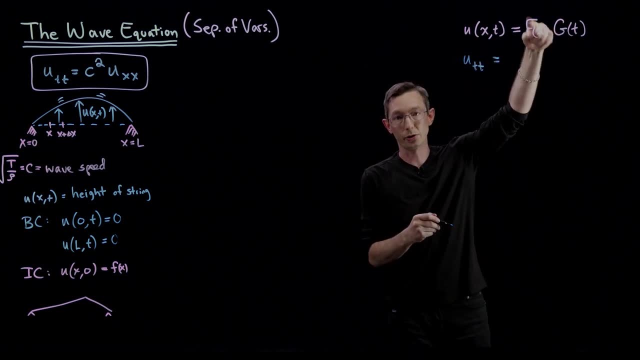 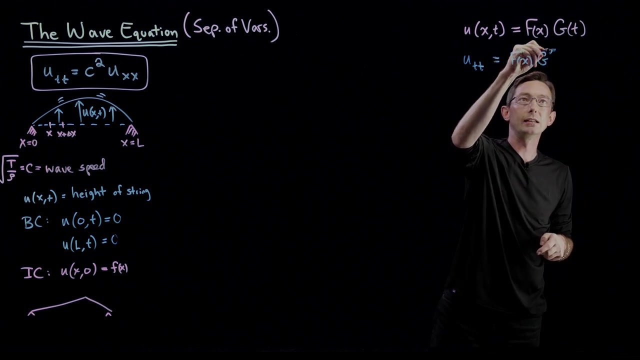 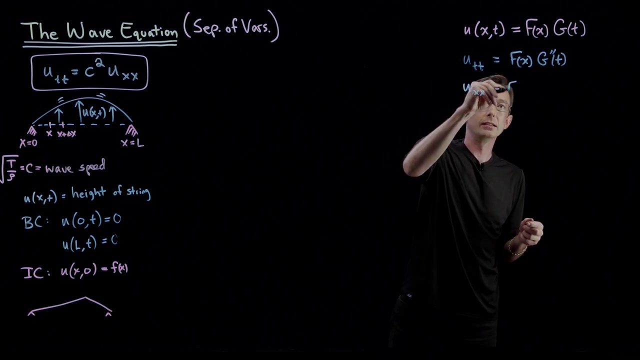 this PDE. So we need to be able to compute u t t and u x x. Pretty simple. So u t t is just the second partial derivative of this with respect to time. So that's, you know, f of x times g double prime t, Good. And similarly u x x is f double prime x times g of t. 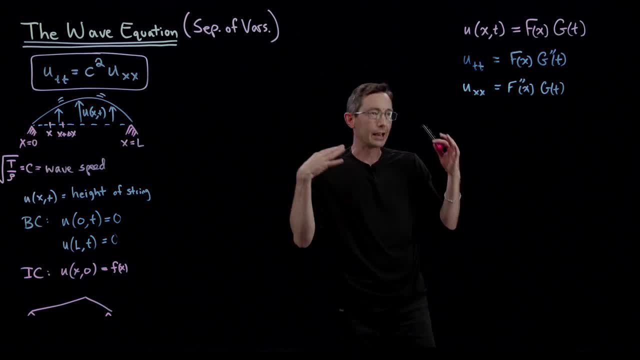 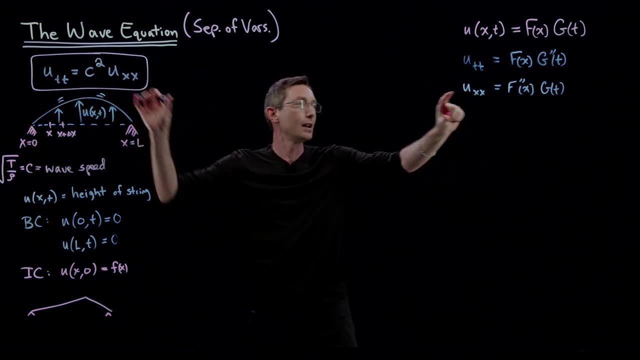 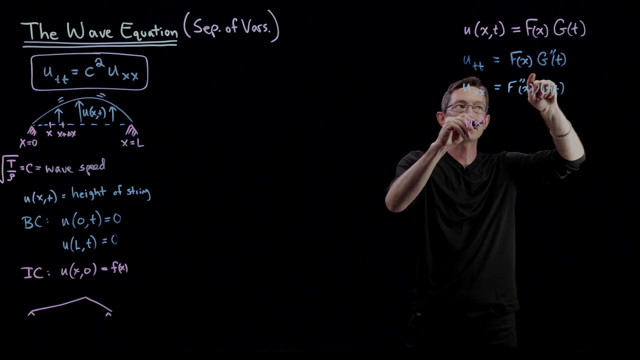 Pretty, pretty simple stuff here, Okay, And because we know that u t, t is just the second partial derivative of this with respect to time. so that's, you know, t equals c squared u x, x. I can use these expressions to essentially say that f x g double. 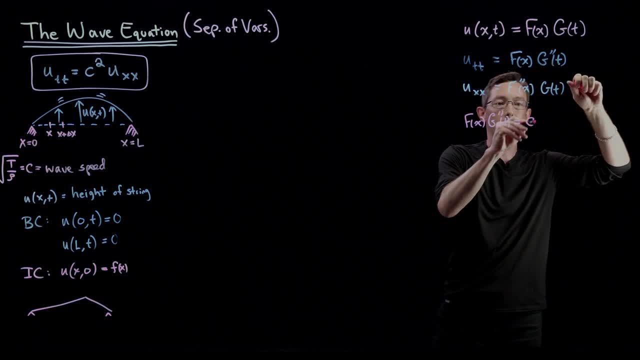 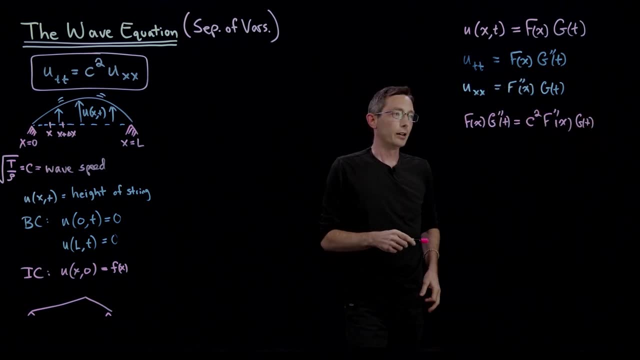 prime t equals c squared f. double prime x g of t. Okay, Good, And so now, just like we've done in the past, what we're going to do is we're going to collect all of the functions of x on one side and all the functions of g on the other side, And we're going to try to turn those. 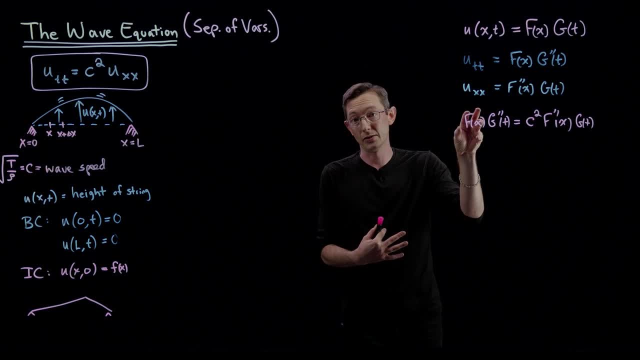 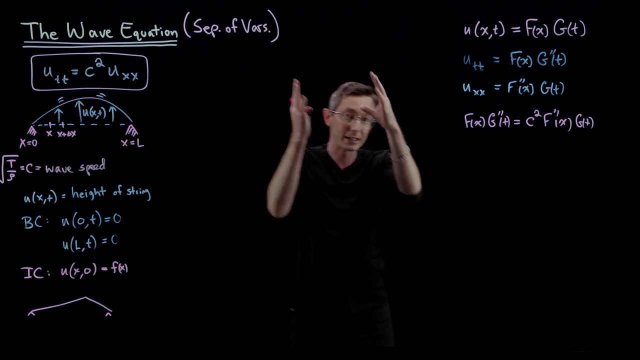 into ordinary differential equations, just of x and just of t. Okay, So we're going to try and take this spatial, temporal problem, this, this, this function of two variables, x and t- and break it down into, you know, just a problem in x and just a problem in t that we can solve using our kind of. 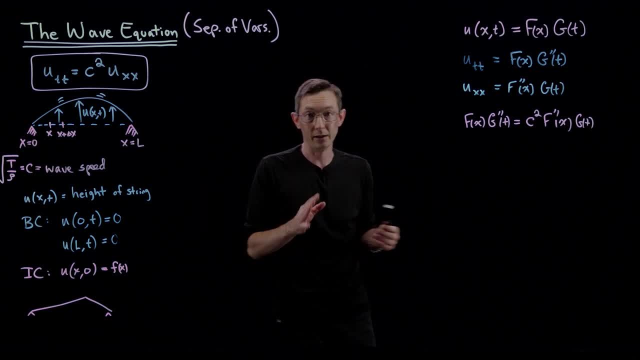 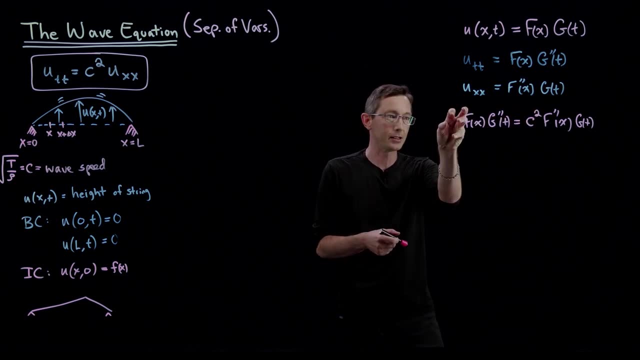 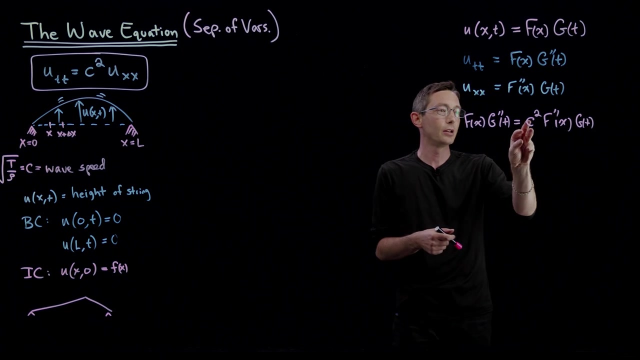 basic ODE technology that we are very comfortable with. Okay, And I always forget. you know where I should keep my c. Should I keep my constant on the x terms or on the on the time terms? I think I'm going to keep the. I think I'm going to move my c's over. So I think what I'm going to do is I'm 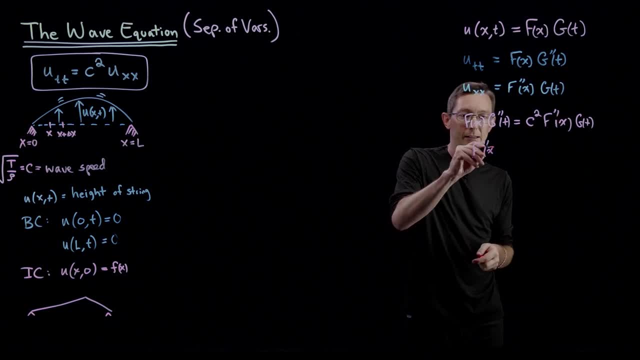 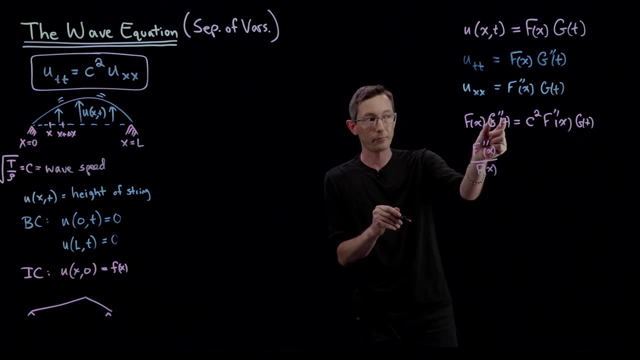 going to say I have f double prime of x over f of x. I'm going to divide both sides by f, I'm going to divide both sides by g And I'm going to divide both sides by c squared, So this equals one. 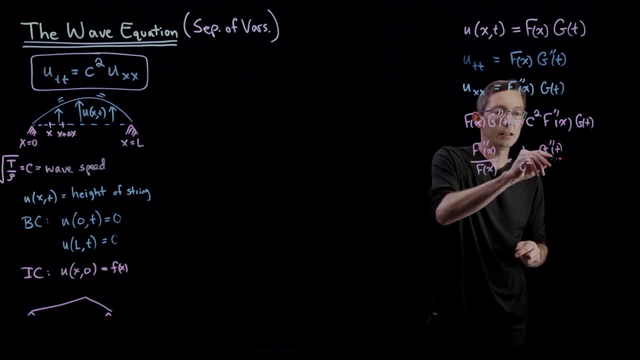 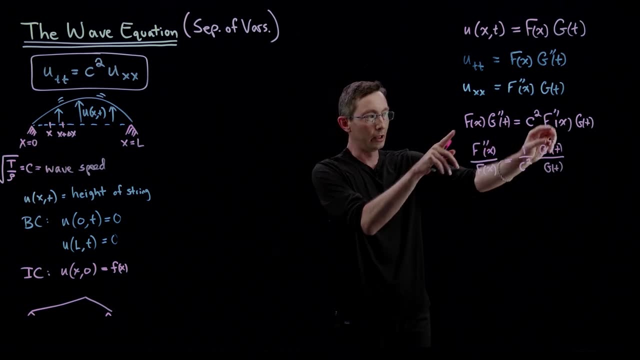 over c squared g double prime, t over g of t. You can, you know, pause the video, slow it down, whatever, But all I've done is I've divided both sides by f double prime, by g double prime, and. 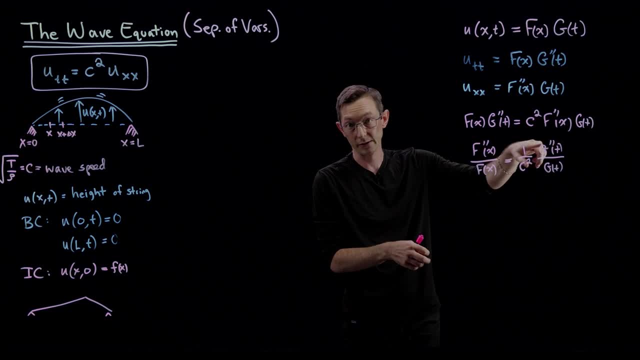 divided by c squared, so that the c squared is now with my functions of time. And this is where, in the last you know video where I did separation of variables for Laplace's equation, I made a really big point of emphasizing that if I'm going to divide both sides by f double prime, I'm going 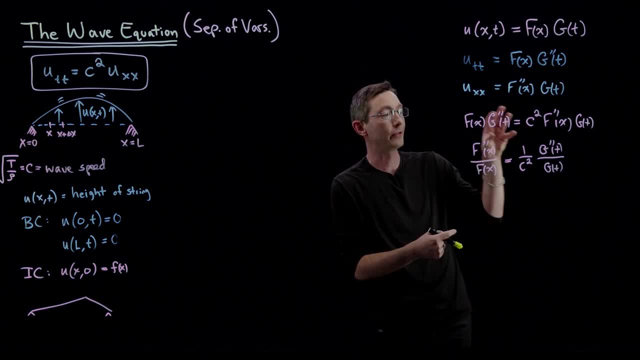 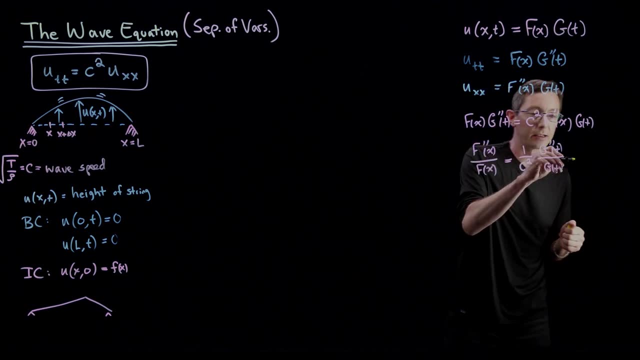 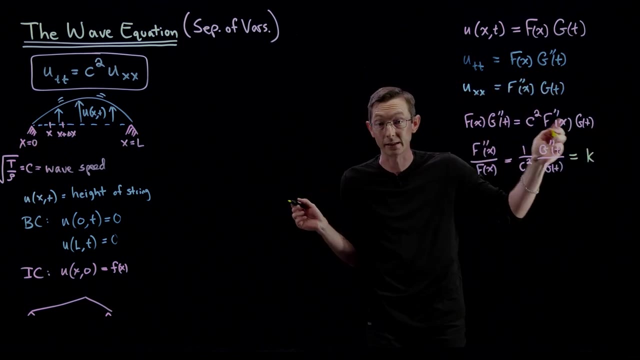 to have a function that's just a function of x and I have a function that's just a function of time and they equal each other, then they both have to be equal to a constant. This has to equal some k, some. you know I should not spell constant with a k, but this is a constant. 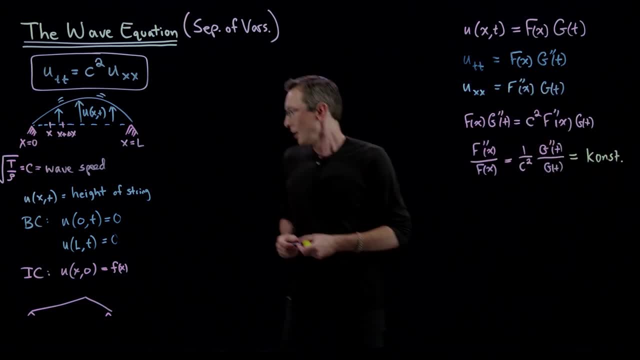 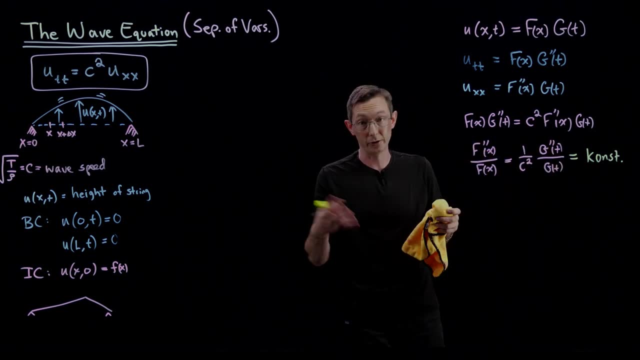 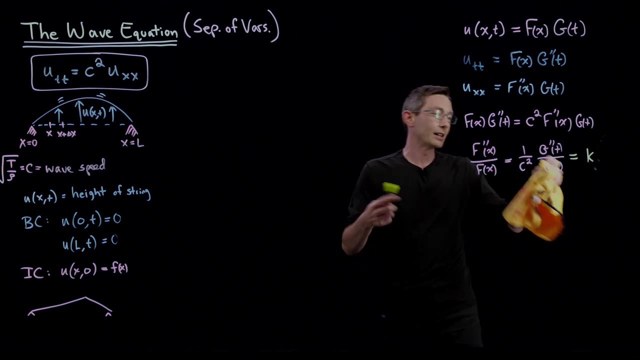 Okay, this is a constant k. Okay so, and that's again, because this is just a function of x and this is just a function of t, and for those to be equal to each other, it has to equal some constant k. And you know maybe what I'll do, because I you know that these 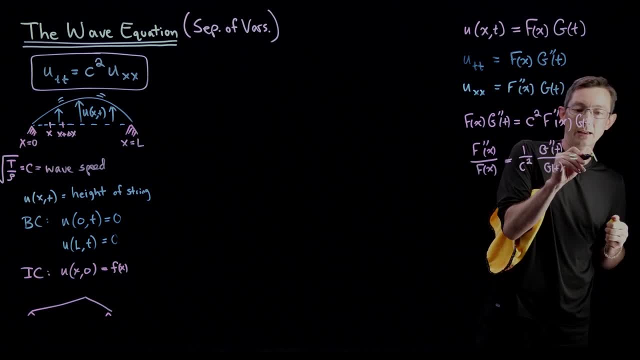 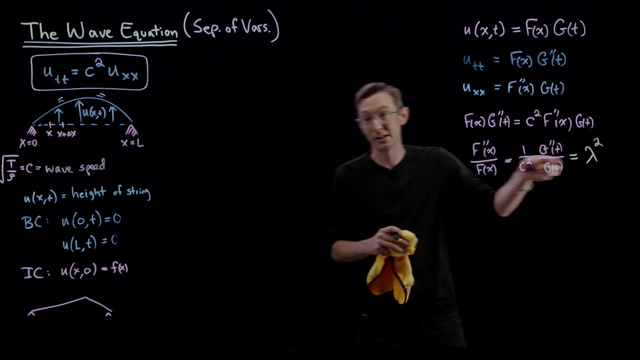 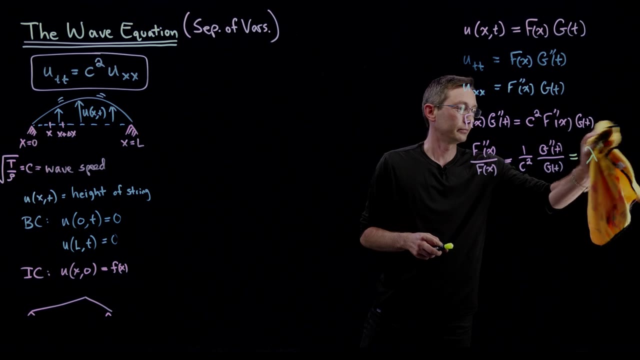 are going to be eigenvalues. I'm just going to call that constant k some constant lambda. okay, some constant lambda, And in fact I'm going to make it lambda squared because I know it's going to be a positive constant. We'll get there. Maybe I'll just call it lambda, Good. 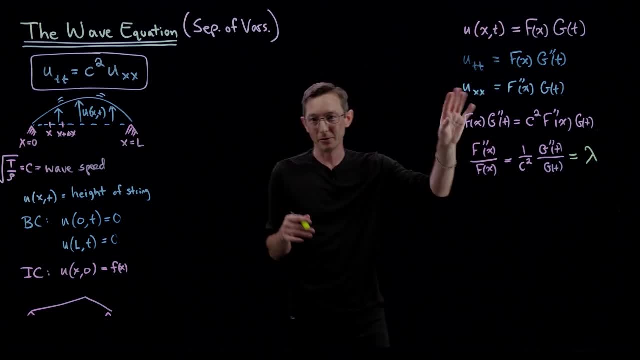 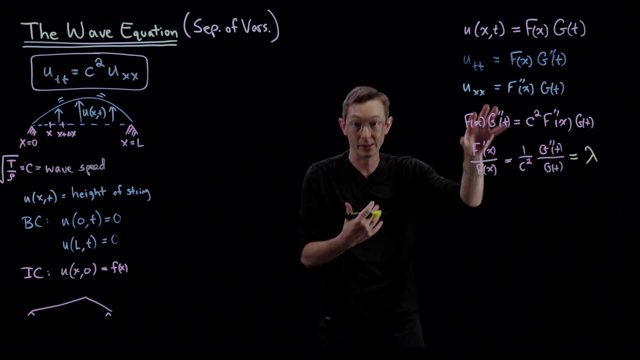 So I should point out- okay, I'll do you know- that the next step is going to be solving, you know, just taking f double prime x over f equals lambda, and solving that ordinary differential equation in x, you know, presumably with these boundary conditions, and then doing the same thing. 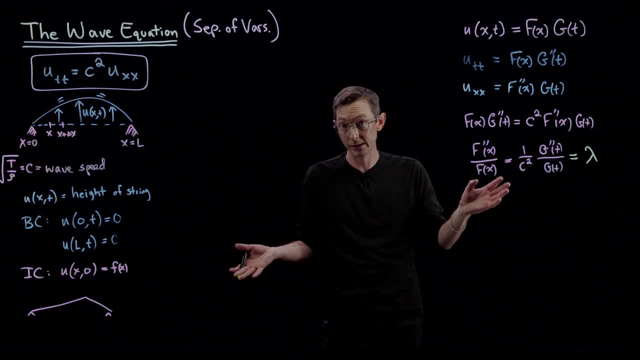 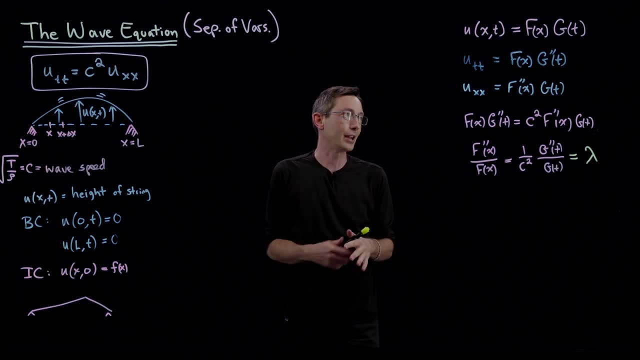 for the time, ordinary differential equation and then combining those. that's what we do in separation of variables. I'll point out you know I mentioned in the last video that the wave equation is something I actually don't usually dive too much into depth in. 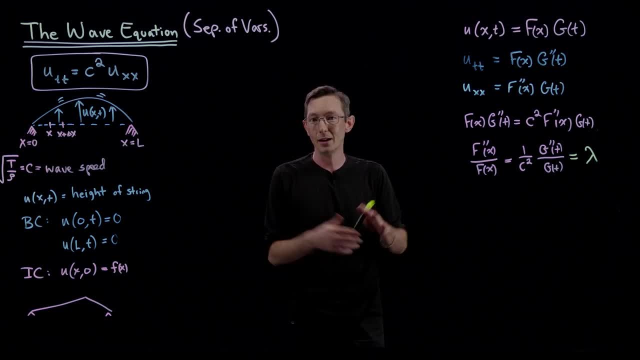 class. It's something you know. I've spent a lot of time over the years contemplating the wave equation. It's never been my favorite PDE that I felt really, really comfortable with. It's super important, It's everywhere And over the last few days I have just been, you know, wandering around. 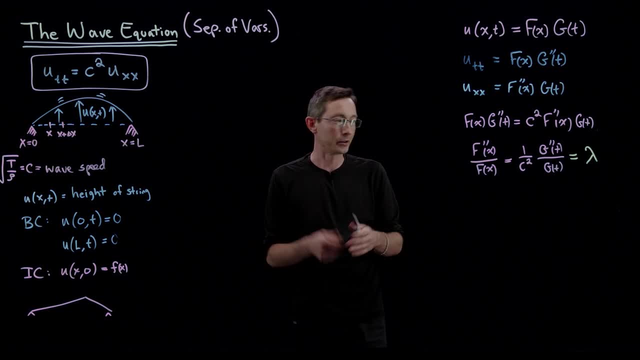 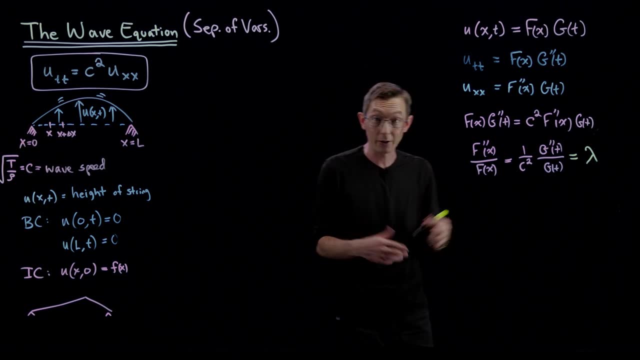 like a planet. Planet means wanderer, So I've just been wandering around, you know, listening to guitar music and thinking about the wave equation and its solution, And when I derived this out as kind of a test run of this video, I got all the signs wrong. My C's were all 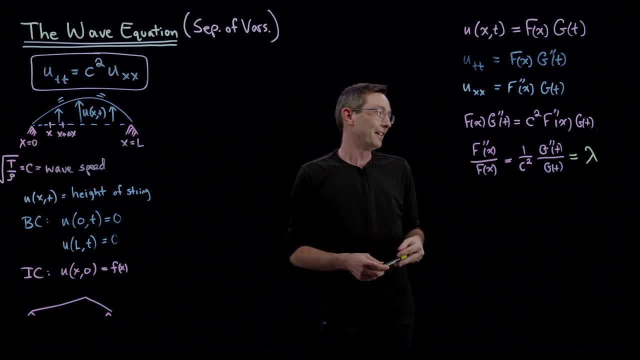 in the wrong place. So I just want you to know that if it looks like well, if it goes really smoothly- it didn't the first time- And if it doesn't go very smoothly, you are forewarned. Okay, this is the kind of thing. you got to be really careful to keep track of the signs and 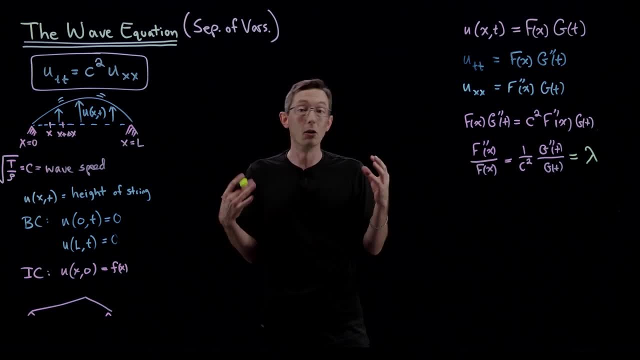 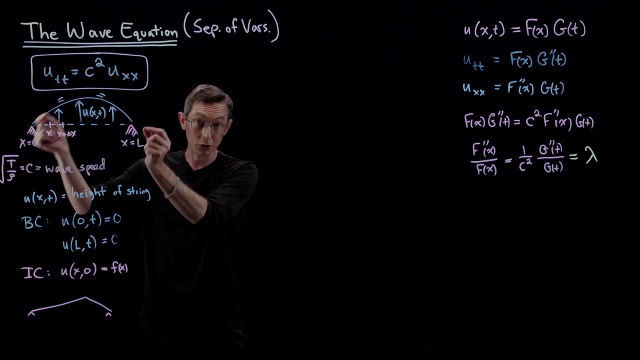 where the C's are And all of that stuff. And for me personally, the only way I can keep track of it is to have some idea of the physical intuition of what I want my solution to look like. So maybe, before I solve this, I'm going to just go back to the physics. here We have a guitar string that's pinned in. 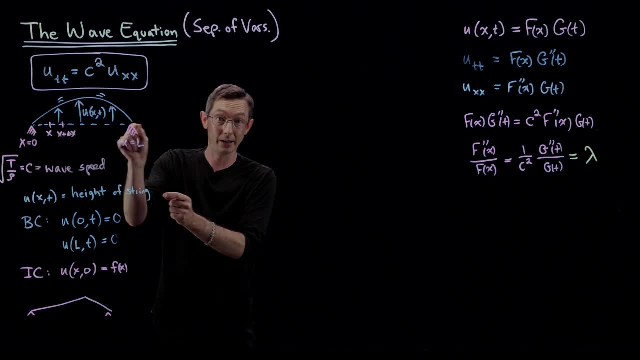 two places at the. you know one condition: X equals zero, and another: X equals L, the length of the string. The only solutions that can satisfy those two boundary conditions essentially have to be the C's. So I'm going to go back to the physics here And I'm going to go back to the. 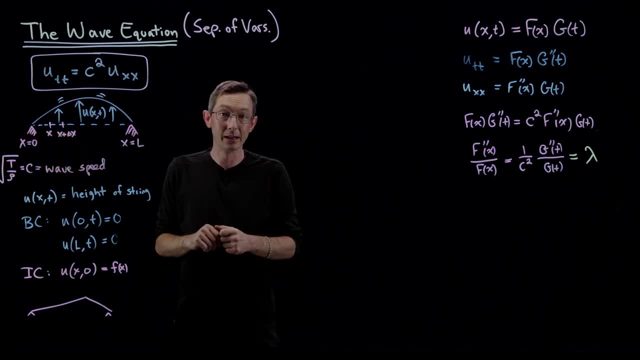 that have you know a period of L, something like sine of you know X pi over L, or sine of two pi X over L, or three pi X over L or four pi X over L. Those are the only you know basic. 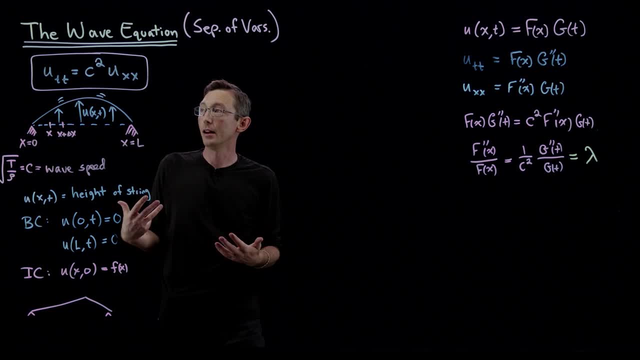 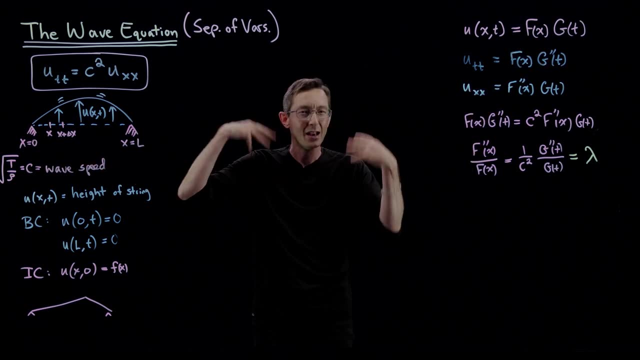 solutions that can satisfy these two boundary conditions. And so I kind of already know that my functions of X, my F of X, are going to be signs with that period, And so that's going to help me figure out should my lambda be equal to zero or not. And so I'm going to go back to the physics. 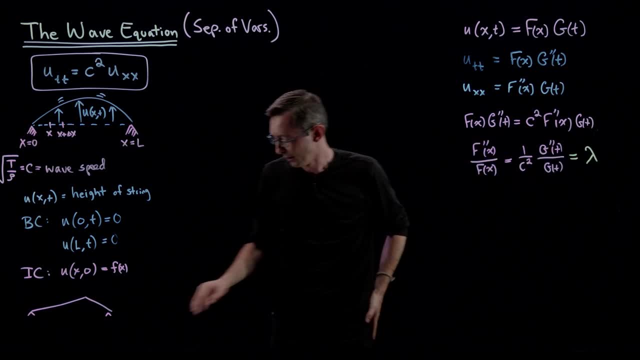 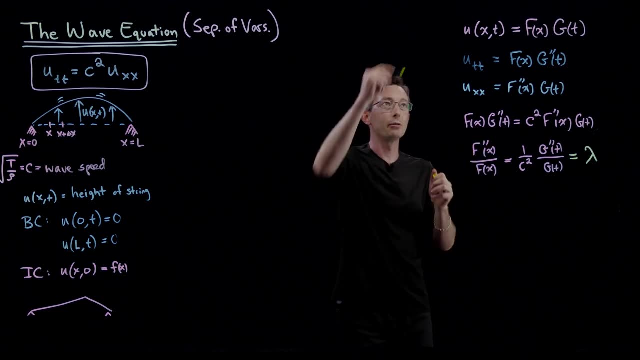 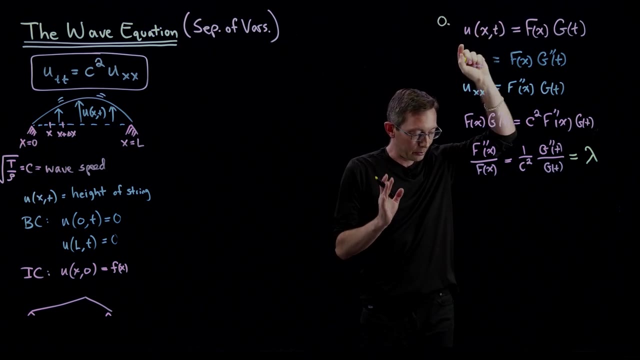 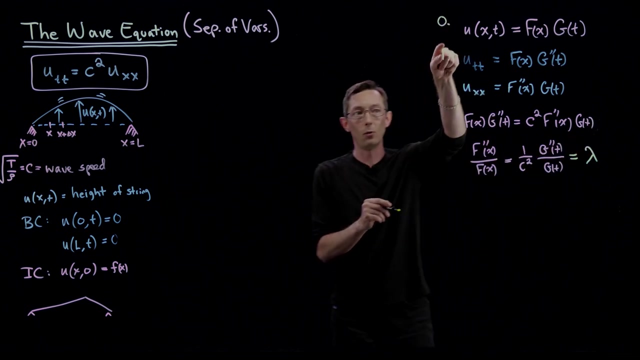 here. I don't know if the is computing all of the derivatives and getting to this point here. So step one is computing all of these derivatives and kind of arriving at this basic expression here. and now step two: I'm going to break it up into two parts. I'm going to solve. 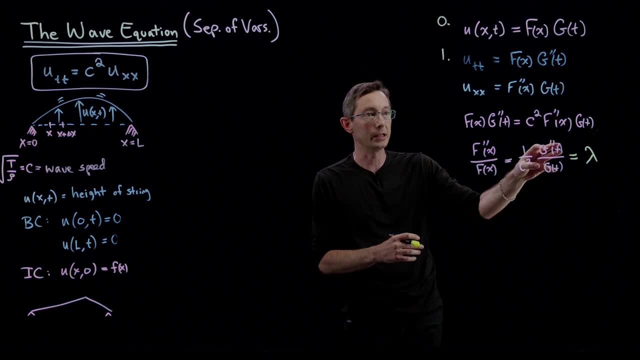 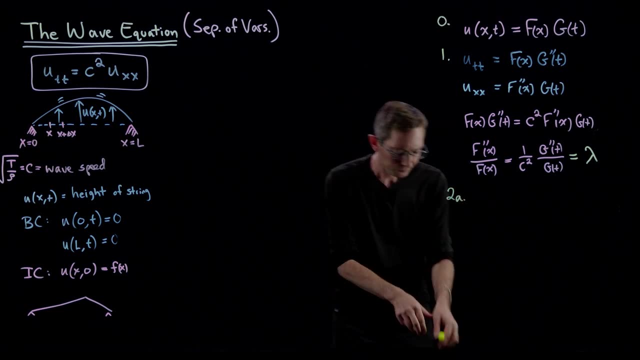 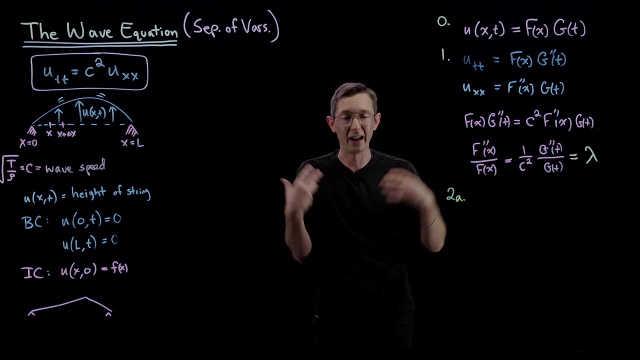 the ode for the functions of x and I'm going to solve the ode for the functions of time. so, and let's call this 2a, because there's two parts to this. what I want to point out is I always want to pick the one that's easiest to solve first, where I have more information. 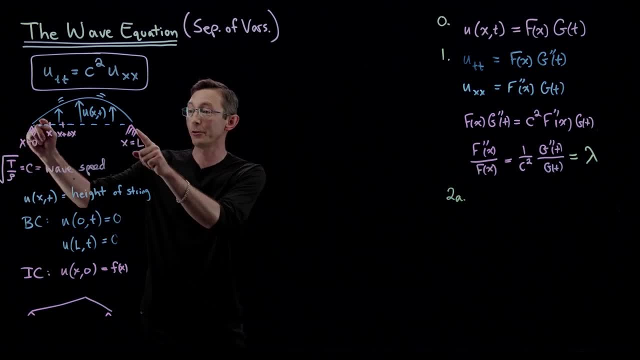 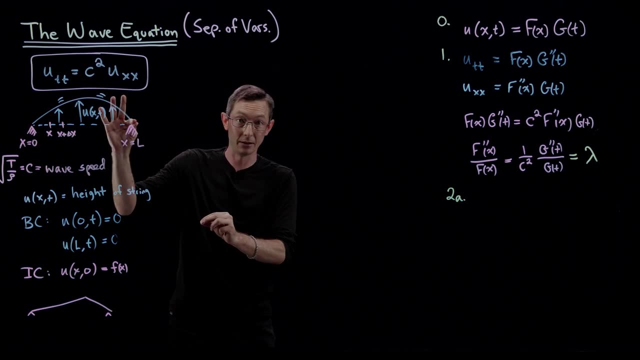 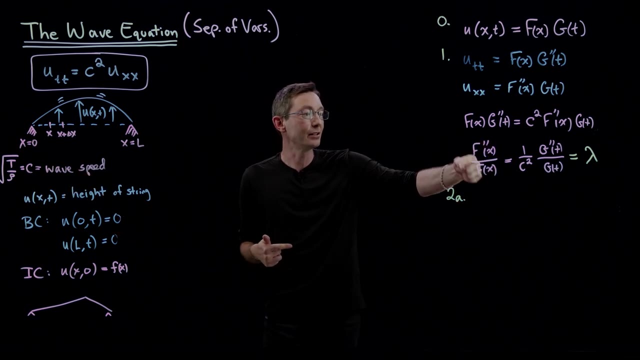 and, if you notice, here it looks like my boundary conditions are pretty simple. I have, you know, fixed pinned boundary conditions at x equals zero and x equals l, and so I'm pretty sure my functions of space are going to be sine waves with that length l period. so I think that it's going to 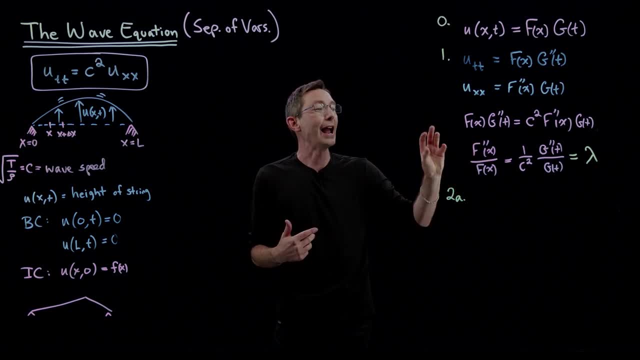 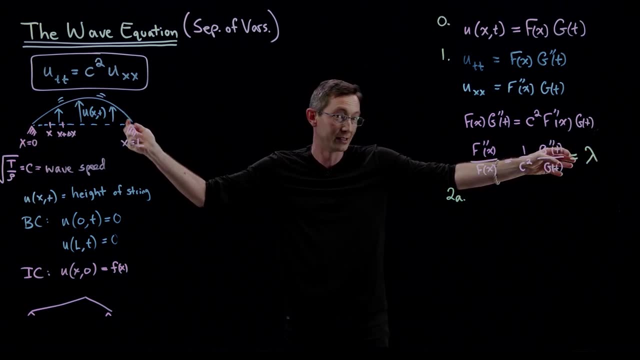 be easier to solve these f equations first and then, once that determines uniquely what this constant is, again, this constant is going to determine, be determined somehow by this length, l. once I determine what that constant is and what these solutions are, then I can solve for how those vary in time. 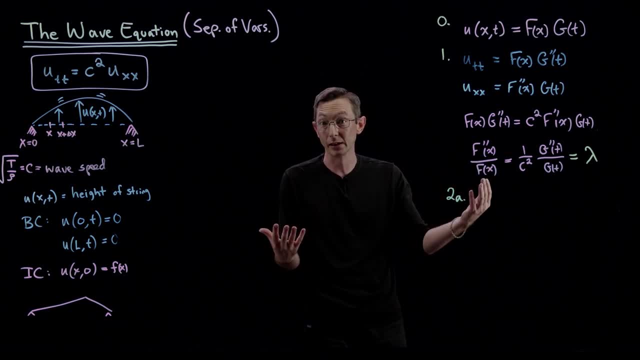 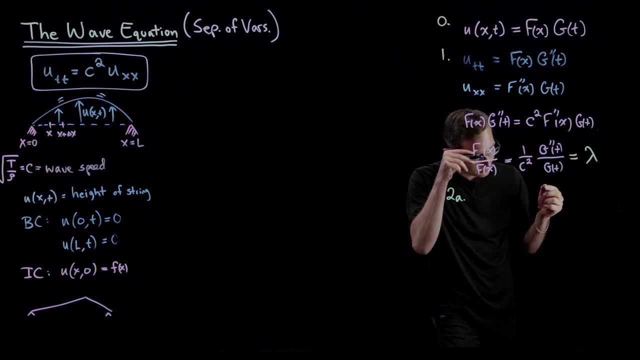 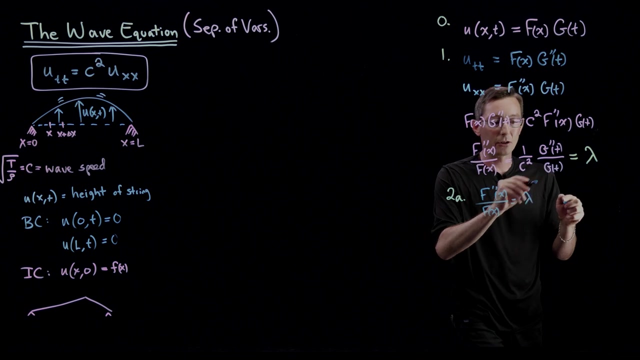 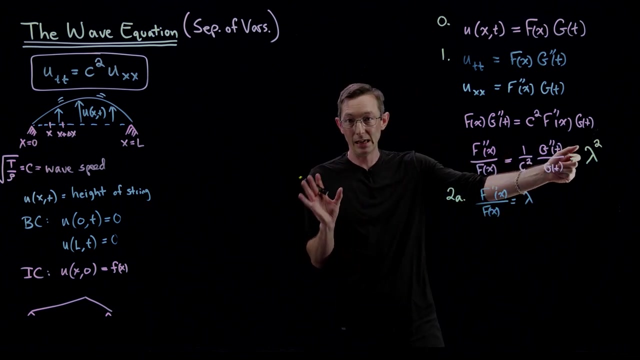 so I'm going to start with my functions. f. that's just, generally speaking, a good idea to start with the easy stuff first. and so here we have an equation that's something like you know: f double prime x over f of x equals. maybe I will call this lambda squared, but I think I think I remember what issue I had when I was. 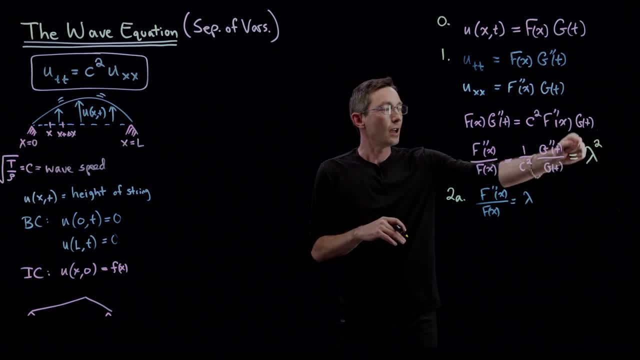 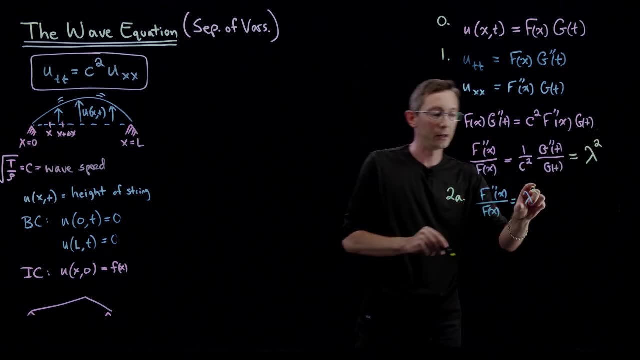 deriving this a couple of days ago is that I am used to this constant being positive, this lambda squared. and when I used a positive constant here, let's, let's say this is lambda squared. when I used a positive constant, I got the wrong solutions to this ordinary differential equation. I'm looking. 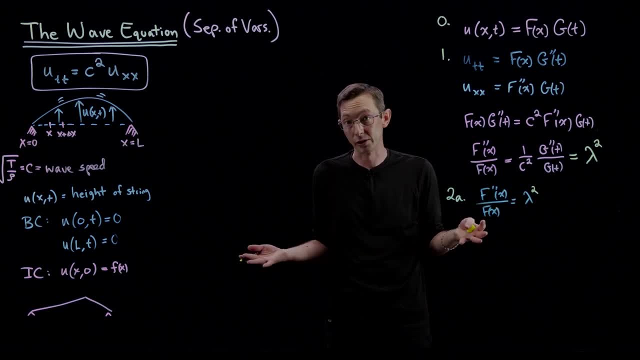 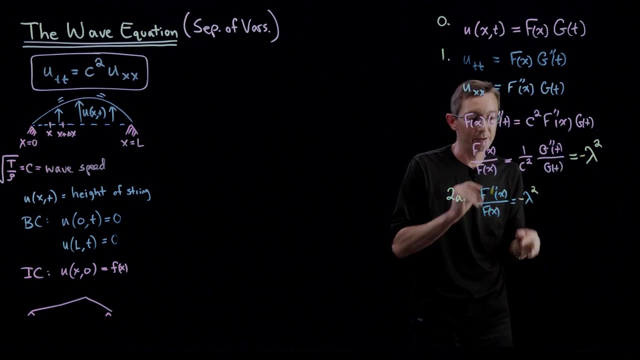 for sines and cosines in x, and I think I got like exponential functions in x, which is not right, and so I had to remind myself this could be a negative constant. this, this constant that both of these equal, this can totally be a negative constant. so this is going to make my life a lot easier and I think 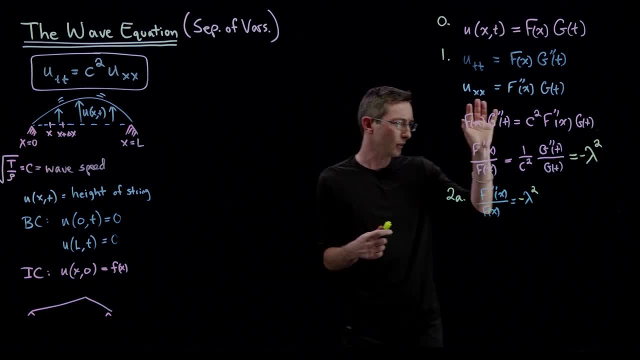 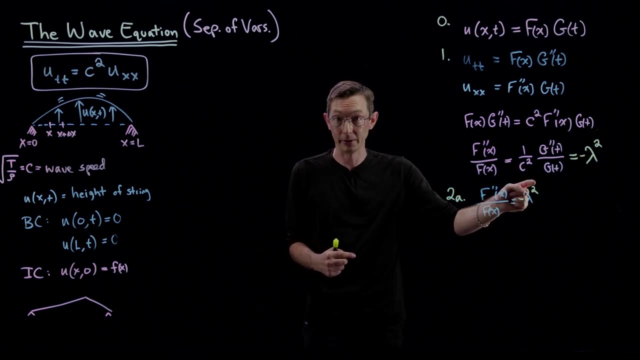 what you, what you should do for those of you at home, is you should try this for a positive constant and work out what those solutions f of X are and convince yourself that you can't possibly satisfy these boundary conditions with the exponential functions you get with a positive lambda squared. 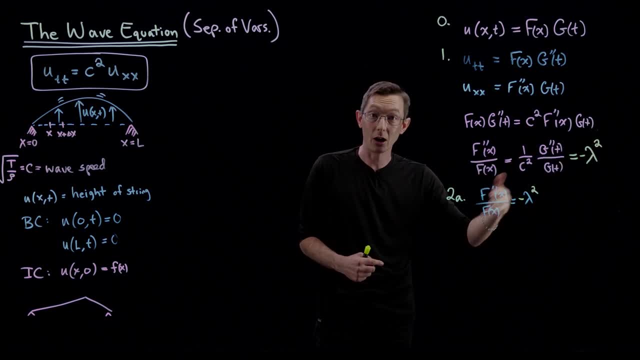 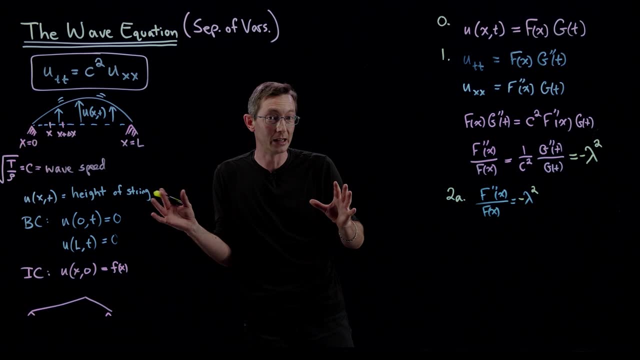 But when you use negative lambda squared, we're going to get sines and cosines out which make it so we can satisfy these boundary conditions. So I'm kind of skipping a couple of minutes of existential crisis for you and we're just going to use the prior knowledge I have. 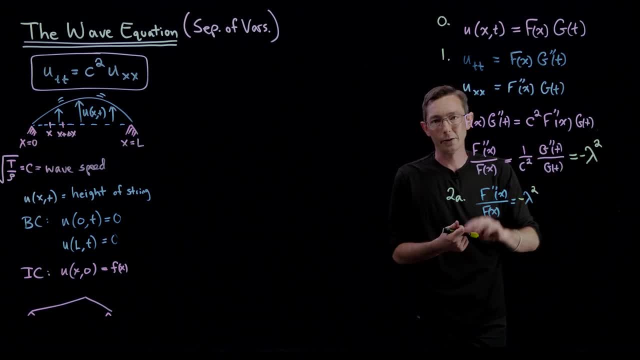 that this should probably be a negative constant, But you can figure this out yourself. This constant at this point is completely undetermined. It can be anything you like, And I'm using lambda squared because this is a second-order equation and it's just going to be easier to have it be lambda squared. 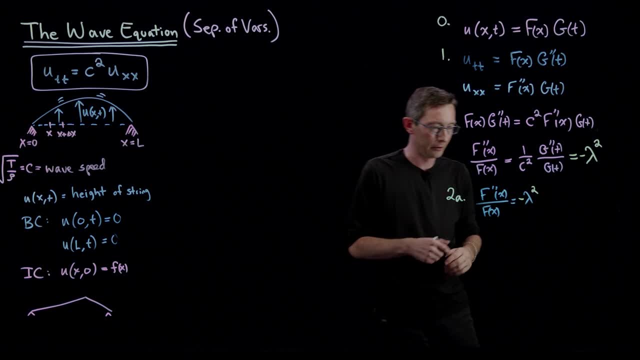 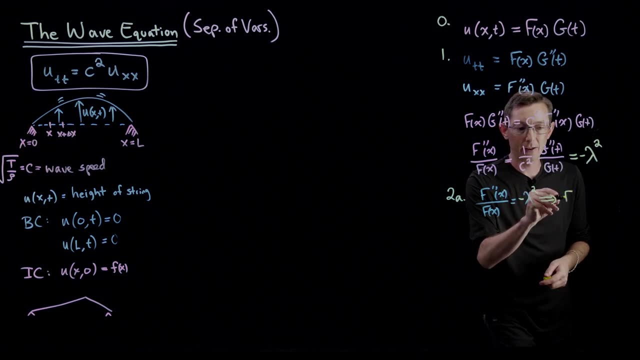 You could just call this some constant k and work it all out yourself. Okay, so what we have here- and we're just going to switch back to yellow- is that we have f double prime plus lambda. squared f equals zero, And since this is not a partial differential equation, 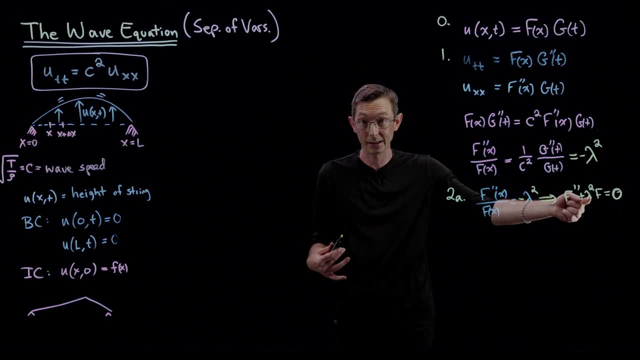 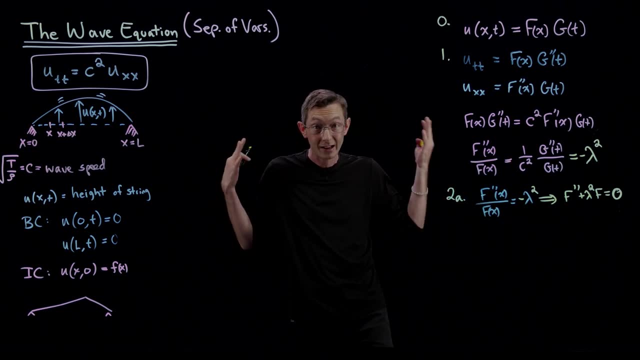 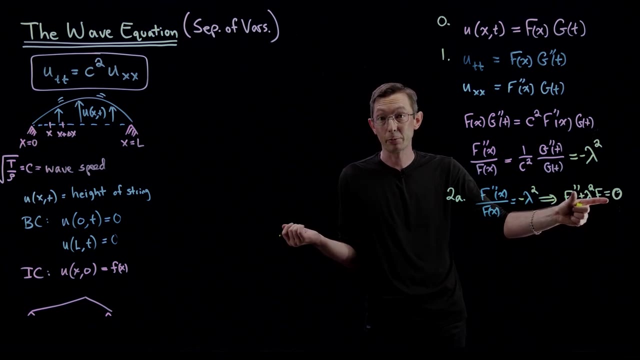 this is an ordinary differential equation. It has one, It's an independent variable, x, And so this ordinary differential equation is easy to solve. We know how to solve second-order linear differential equations. This is essentially the equation for a mass on a spring. 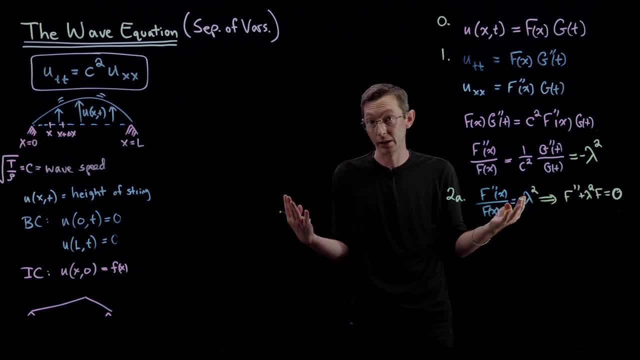 And this lambda squared is the square of that spring frequency, the frequency of oscillation. So that's again why I needed this to be negative, so that when I multiplied f and added it I got a spring equation that has a plus and minus. 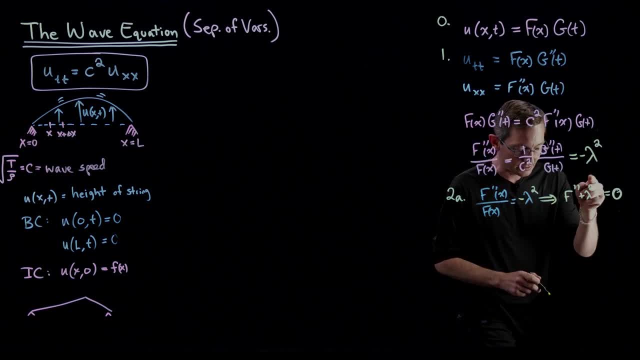 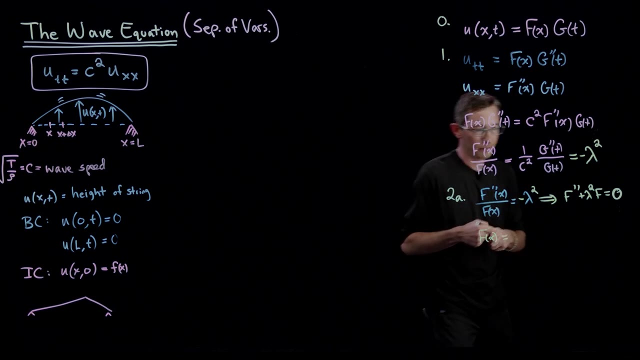 So that's my omega eigenvalue, okay, And so essentially, we know that this is going to have solutions: f of x equals. and how do I want to write this? This is going to have f of x equals, some constant. I'll call it alpha. 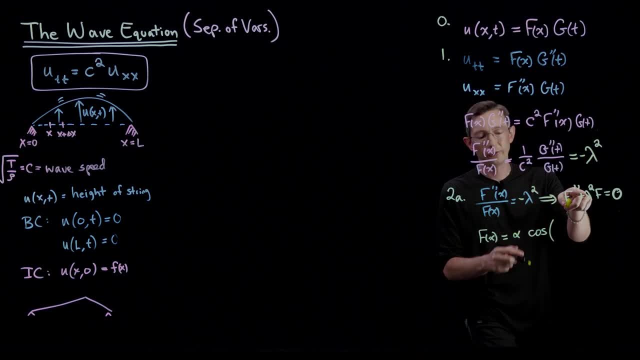 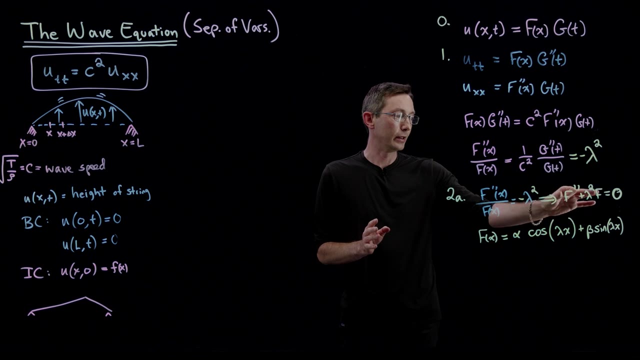 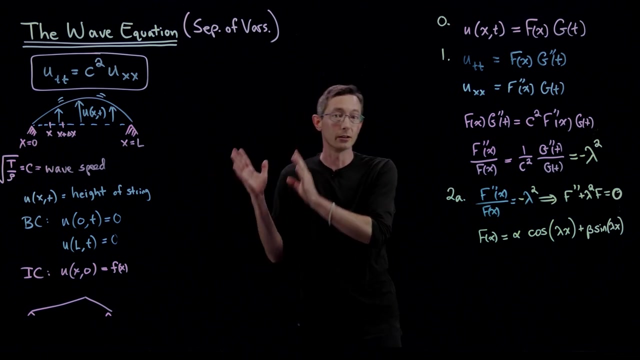 cosine of lambda x plus some other constant beta sine lambda x. Okay, good, So this is just what happens when you solve this differential equation: You've got a cosine and a sine component. Again, you can go back to your kind of basic linear. 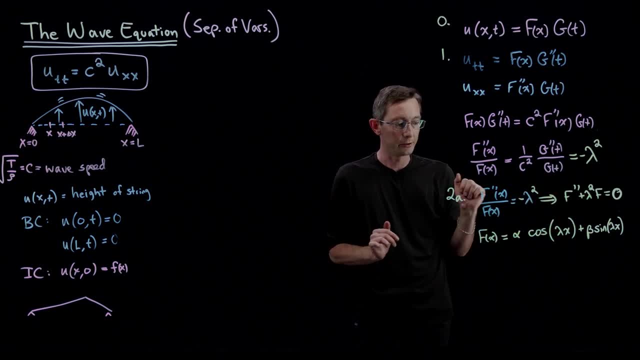 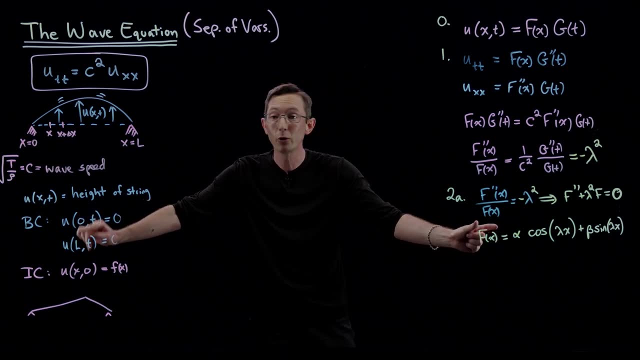 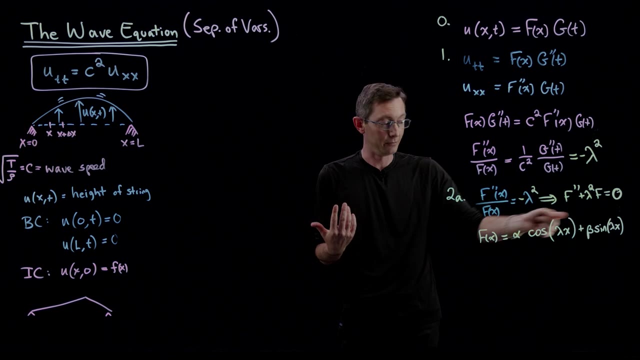 ordinary differential equations to solve this. This is the solution, And what we know is that the only way that this function f can satisfy both boundaries, f can satisfy both boundaries, the boundary conditions being zero, at x equals zero and x equals l, is essentially- you know, cosine is not going to be ever zero- at x equals zero. 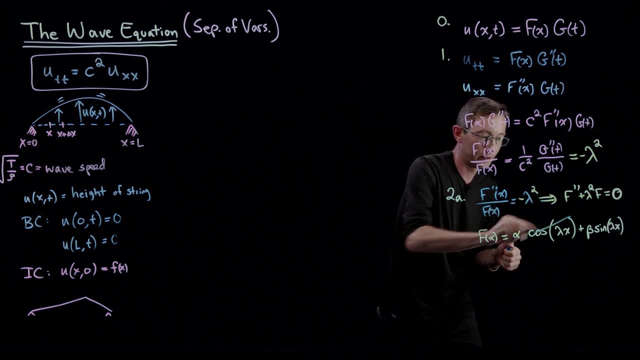 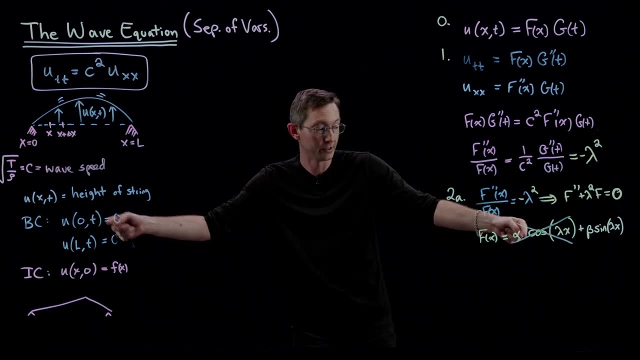 So the only way we can solve this is to have the alpha- all of these terms- equal to zero. no cosine part, because cosine of zero is always equal to one. Okay, so it can't satisfy this left boundary condition unless alpha is zero. 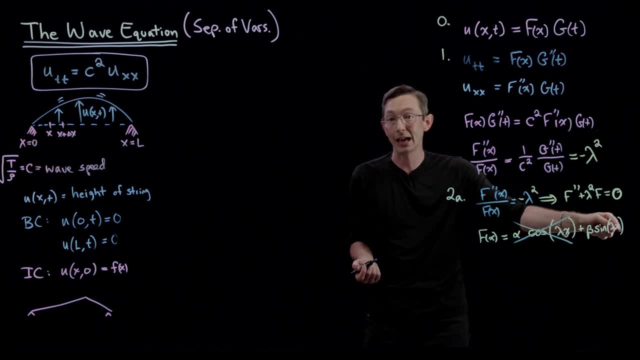 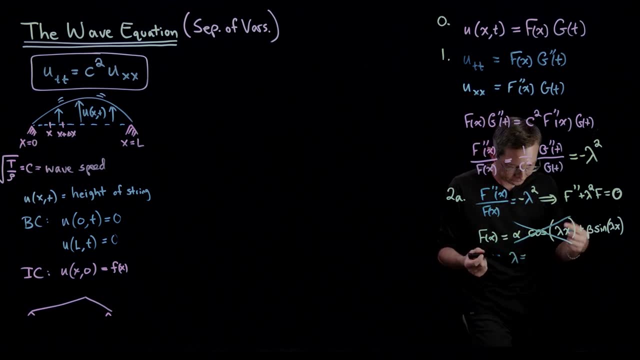 And the only way that sine of lambda x can satisfy this boundary condition is if lambda equals pi over l times some integer n, where n, you know, equals one, two, three, dot, dot, dot. It could also equal zero. 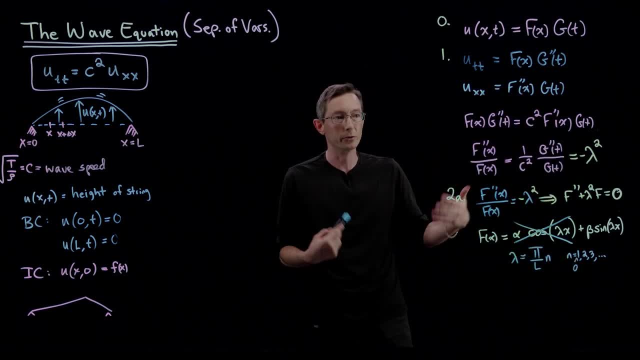 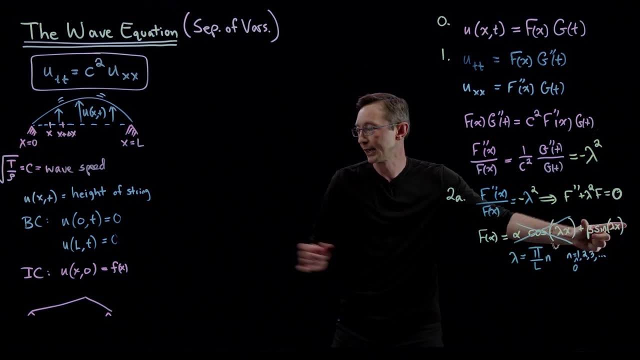 Let's put zero in there. It could be zero one, two, three, dot dot dot. It could also be negative one negative, two, negative three. That's all fine, But the only way that this can satisfy the zero boundary conditions. 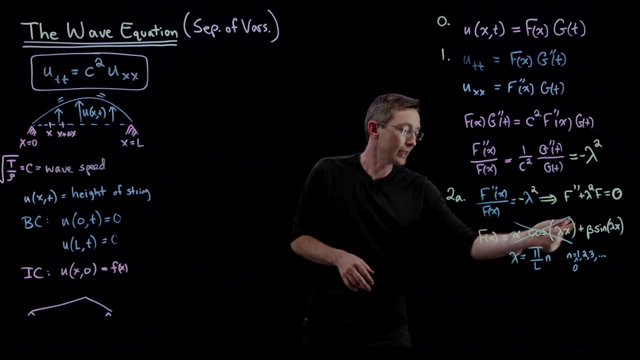 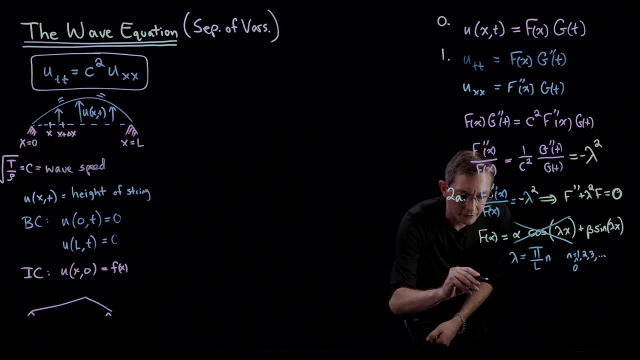 that x equals zero and x equals l is, if lambda equals pi over l times some integer, Okay, And so essentially what we get is that f of x, f of x equals. let's just call this beta n, because there's going to be a constant for every integer n. 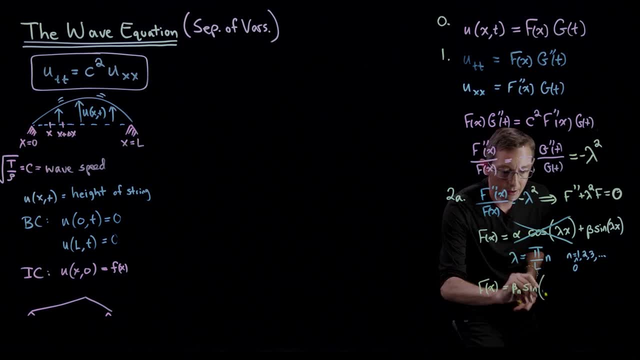 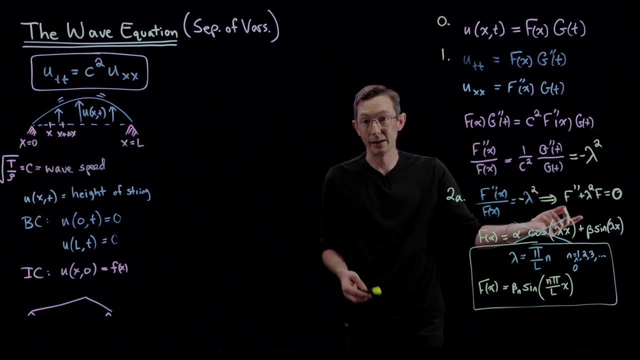 beta n sine of n, pi over l times x, where you know lambda equals pi over l, pi over l times n. Okay, good, So we have solved kind of half of our ordinary differential equation. So we've solved the functions of x. 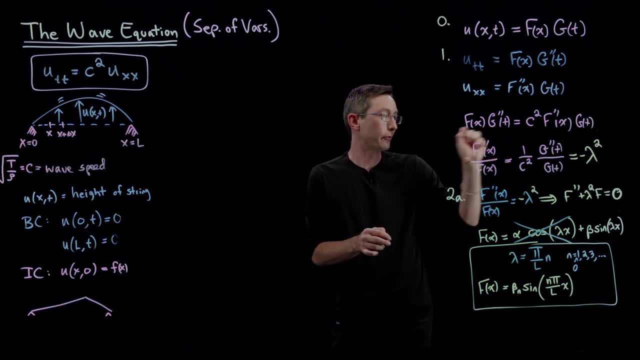 The only way they can satisfy these boundary conditions is for very particular lambda. Remember, special values are eigenvalues, So these lambda are eigenvalues of this ordinary differential equation: f, double prime, x plus lambda. squared f of x equals zero. This ordinary differential equation has eigenvalues, plus and minus. i lambda. 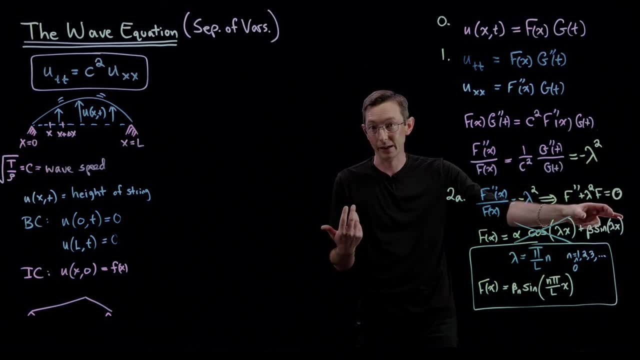 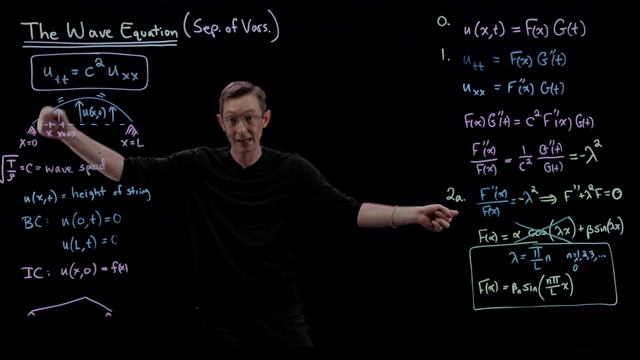 and that gives cosine of lambda x plus sine of lambda x type solutions. The sines are the only ones that can satisfy the pinned boundary conditions here, and they can only satisfy it for very special lambda, for very special values, so that that sine is equal to zero at x equals zero. 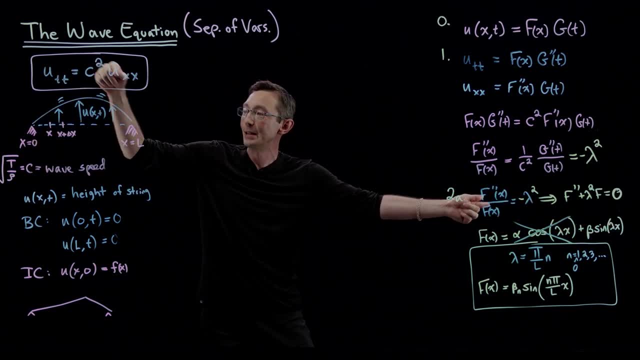 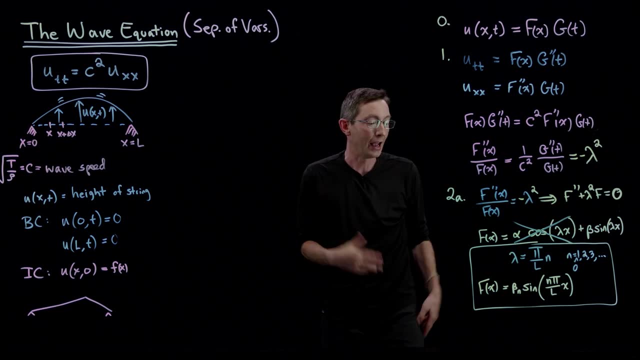 That's true for any lambda. But for it to be equal to zero at x equals l, then lambda l, sine of lambda l, has to equal zero, and that has to be sine of lambda l. you know, has to be some integer multiple of pi. 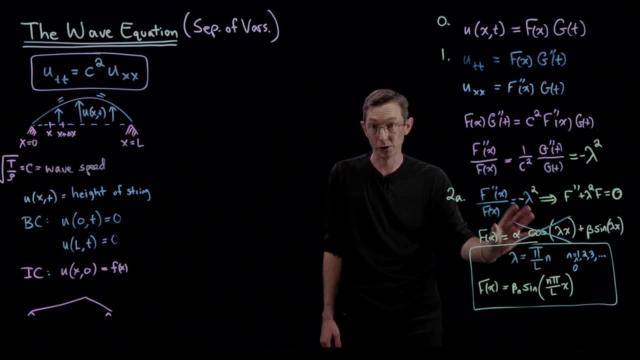 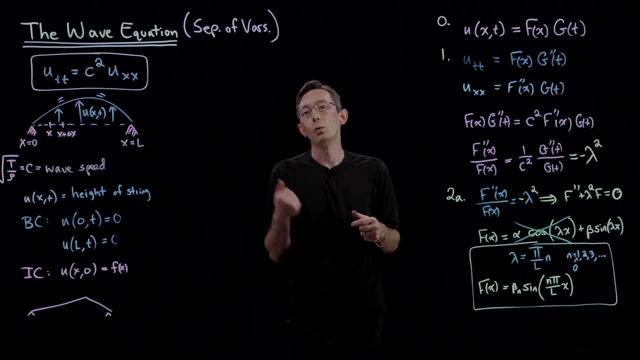 Okay, And so essentially, this is the solution for all the functions in x. Good, And so we've done two solutions. We've done two super important things here. in this step, We have determined that the only spatial solutions to this partial differential equation 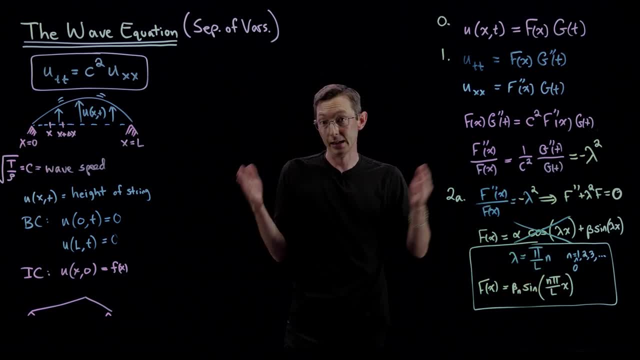 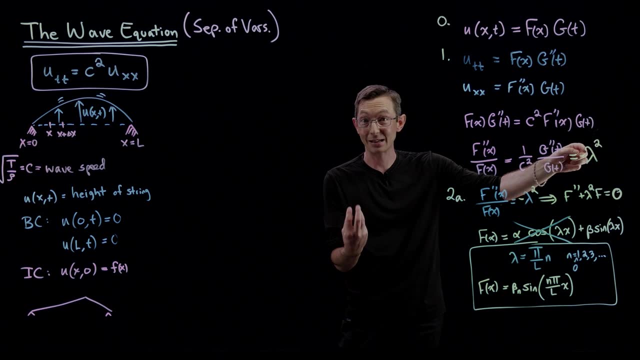 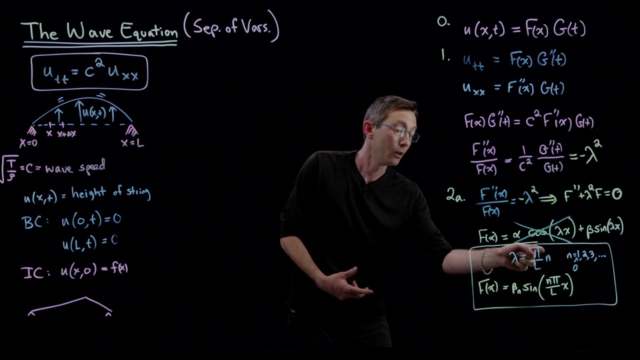 can only be built out of sine functions in x and we've also determined out of all of the possible constants that these could equal. lambda has to be a very, very special constant, an eigenvalue constant given by pi n over l. 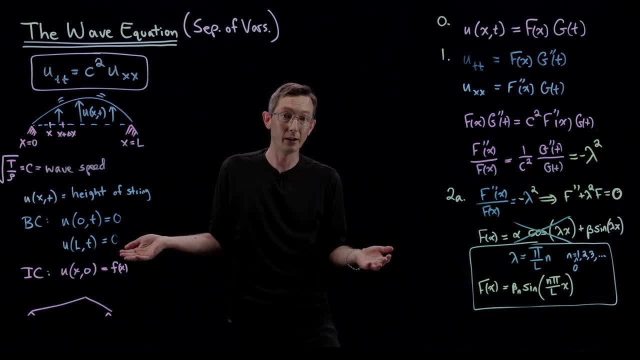 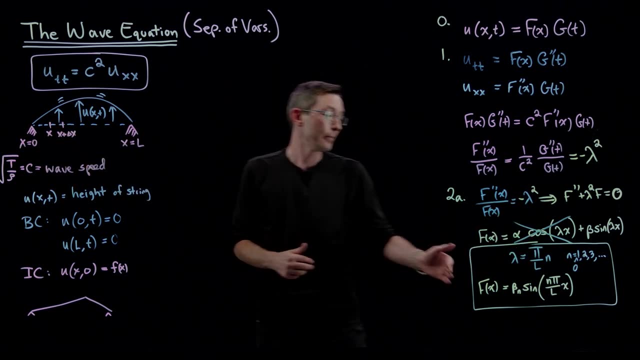 where n is an integer and l is the length of my string. So we've determined that our eigenvalue has to be pi n over l to satisfy these boundary conditions and that our functions of x are sines. you know, with that frequency, 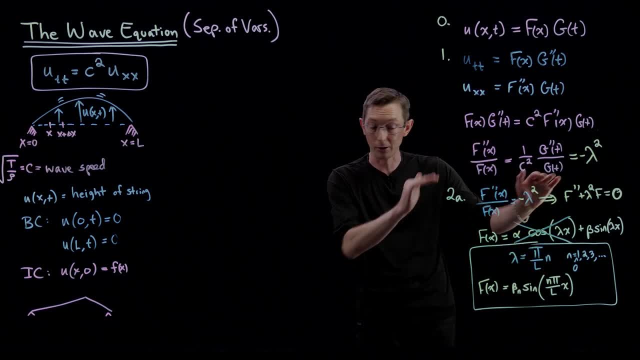 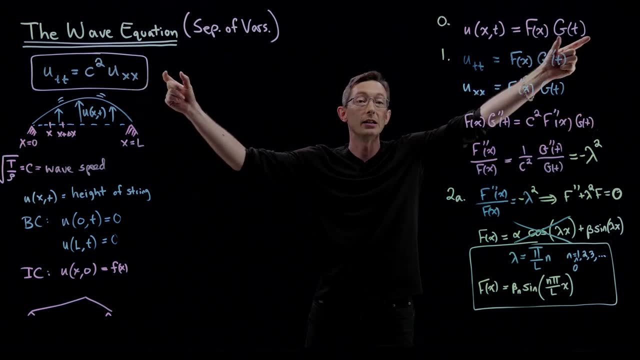 Good. So that was believe it or not. that was the easy part. And now for 2b, we're going to solve the same equations in g for the temporal dynamics for these g of t coefficients here. So let's do that. 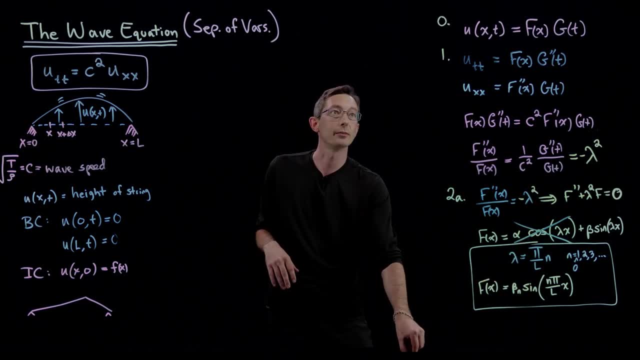 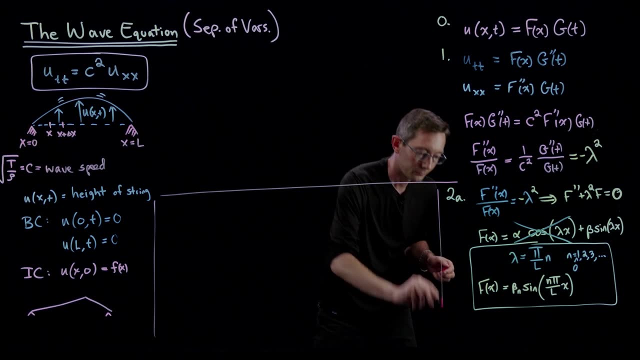 And actually this one's not going to be super hard. now I just want to make sure I give myself space to do it, So maybe I'll just do it right here. So for 2b, we're going to be solving now my g equations. 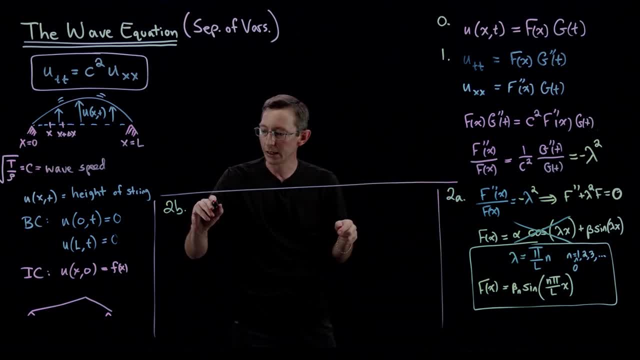 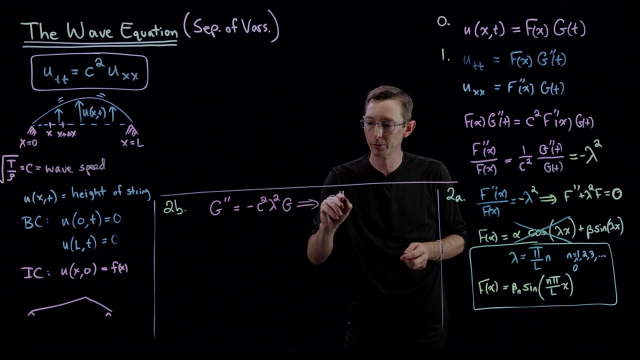 which are going to be something like g double prime equals minus c squared lambda squared g. Okay, And if I rewrite this, I can say that that's g double prime plus c squared lambda squared g. Pretty simple, Okay. 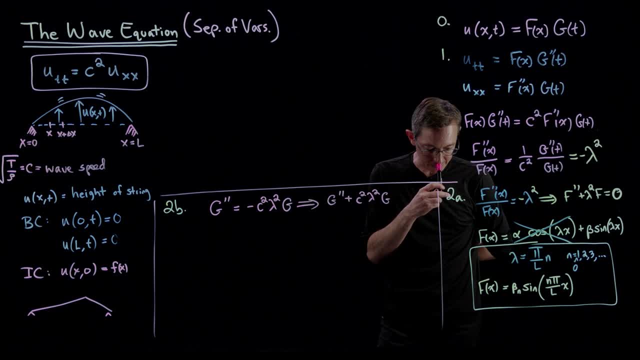 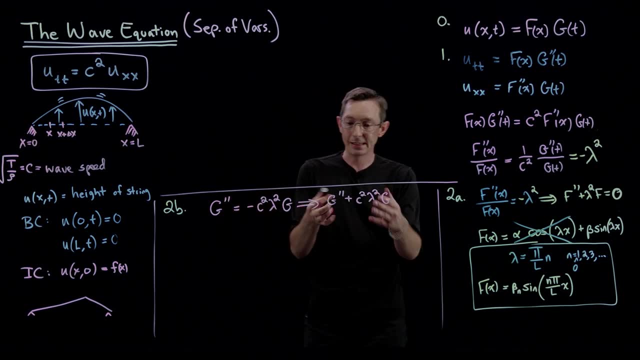 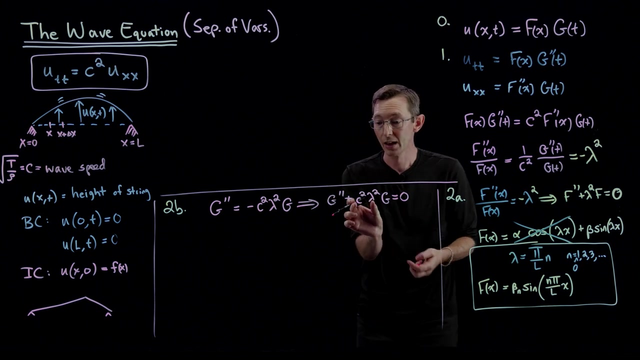 And now this is kind of nice because, Okay, this is. this equals 0.. This is basically the same type of equation. This is also an ordinary differential equation that has the same form as a mass on a spring, And now, instead of the frequency being lambda, 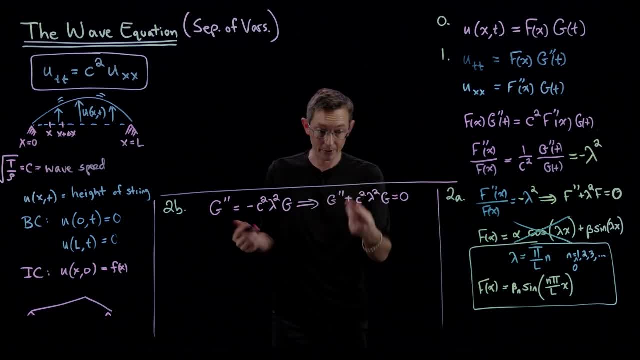 the frequency is c times lambda here, Okay, So, similarly, my g of t's are going to be equal to some, you know, some other constants. I don't know what to call these. Let's call them, I don't know, k. 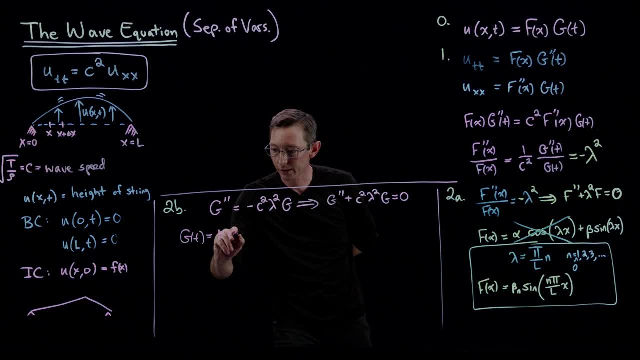 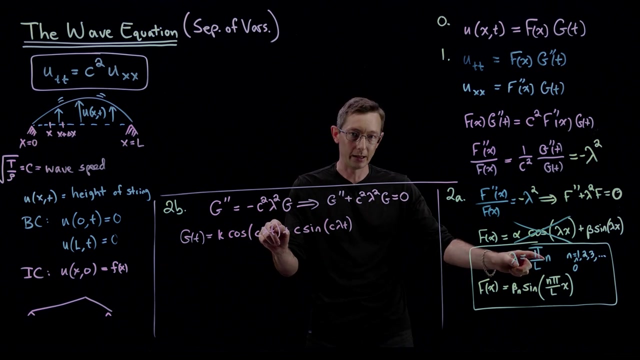 um times cosine of c lambda t, plus some other constant c times sine of c lambda t. Okay, Good, Now um we can essentially fix this lambda. We know what lambda equals: It's pi n over L. So this is, you know c times pi. 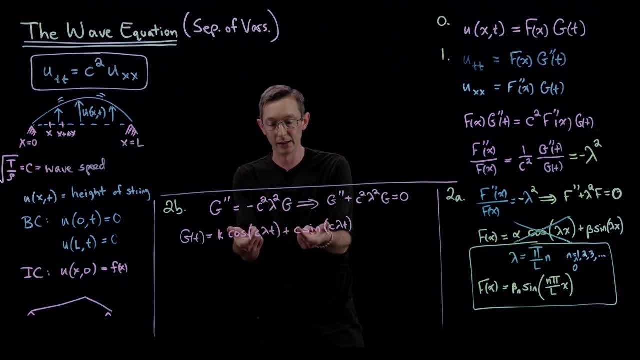 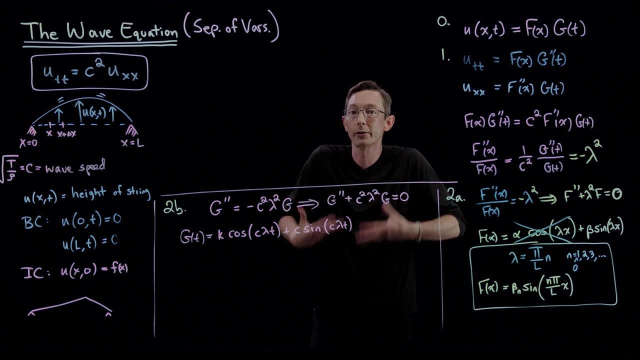 times n over L times t. That's going to be like the frequency of how this string is oscillating in time And again. if I pluck a guitar string, it's generating acoustic waves based on its oscillating frequency. So this frequency here. 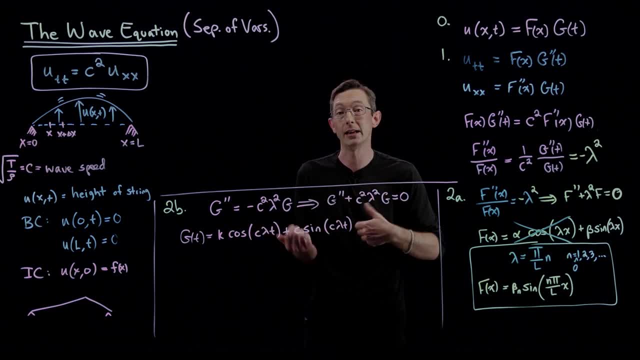 is going to be directly tied to the frequency that I hear when I pluck a guitar string. So it's going to depend on, you know, this c and on this lambda, which is a function of the length of the string, and n, which are the harmonics. 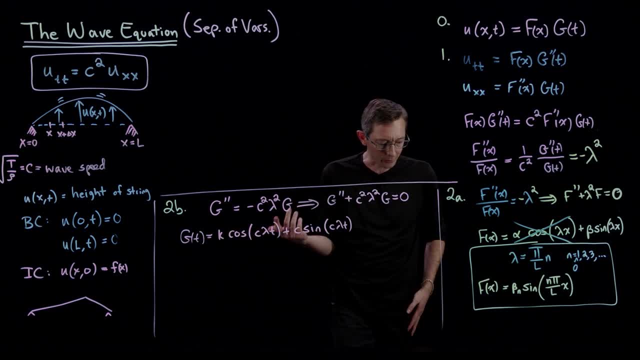 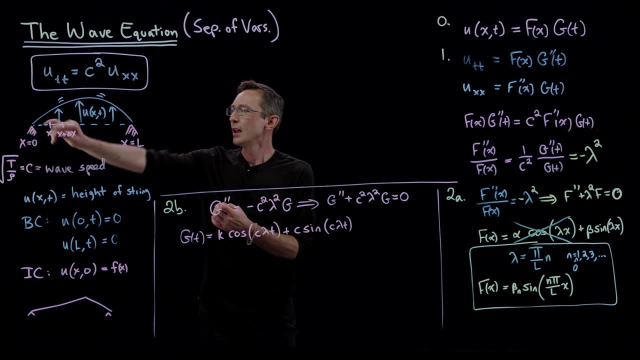 So we'll get to harmonics in a minute. And so now, how do I figure out if this is cosine or sine or some combination? And I think what I would argue is that because this thing starts with an initial condition, u of x comma 0, at time t equals 0,. 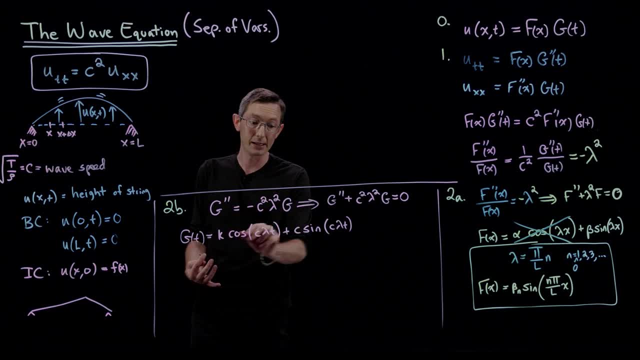 I'm really only considering the cosine portion of this, because sine of c lambda t is equal to 0 at time 0. So I'm only going to use the cosine portion of this to determine my to satisfy my initial conditions. So I'm only going to be looking. 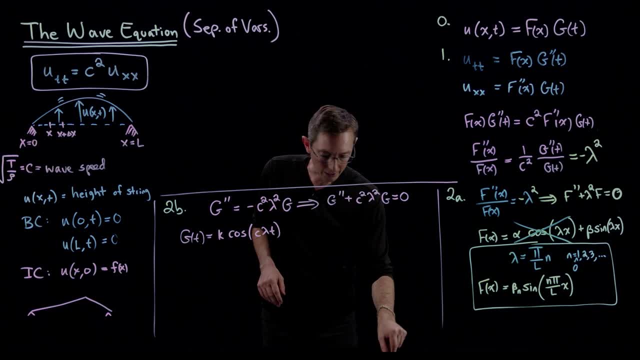 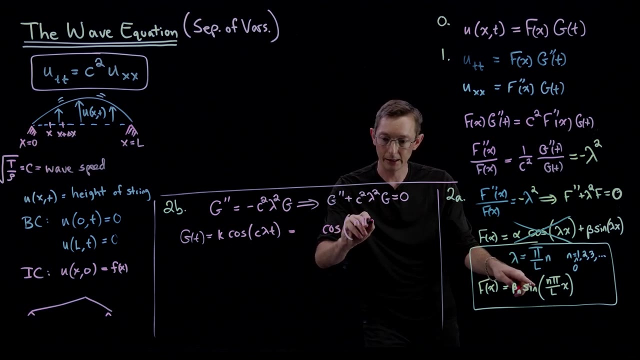 at this portion And I'm going to explicitly plug in my lambda here and I'm going to say this: equals. you know, I've got my cosine of n, of n, pi, c over l, t And this constant k. I'm going to say that: 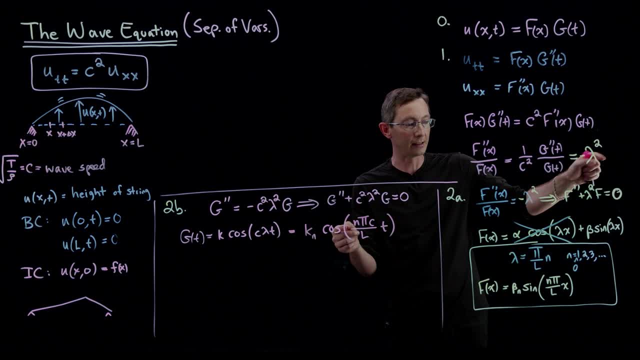 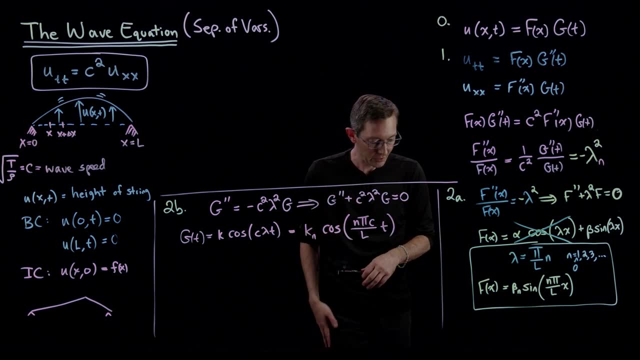 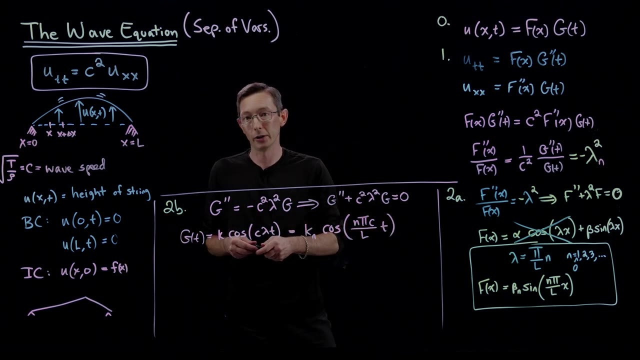 there are n of these constants for every integer n for each of these lambda n. For each of these lambda n, there is a constant outside of that cosine Good, And, if you like, this constant is basically going to be determined by this Fourier transform here. 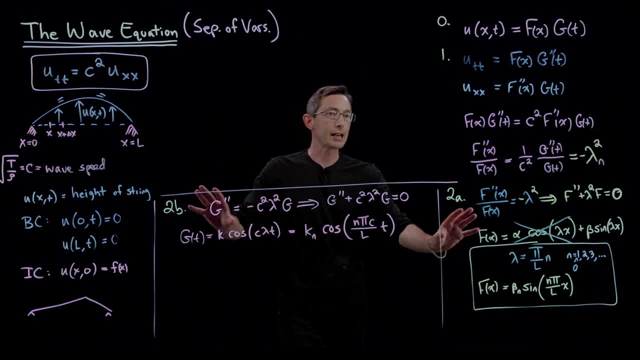 So I'll get back to that in a minute. Okay, so this actually ended up being simple. Now that I had fixed this lambda from my functions of x, I use that lambda in my functions of in my ordinary differential equation for my function of time. 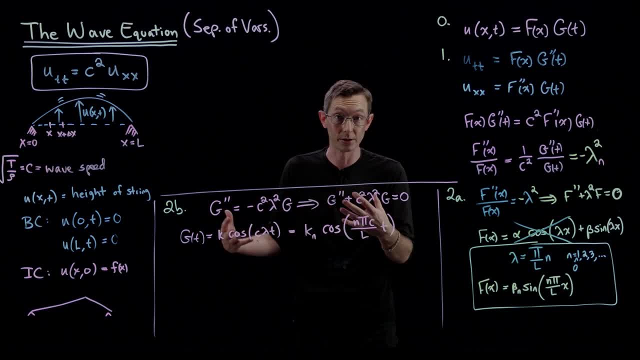 I solve it out. I get that it also is sines and cosines, And the only way I'm going to be able to satisfy this initial condition at time zero is through these cosine components that I have here. And so now, if I combine these two equations, 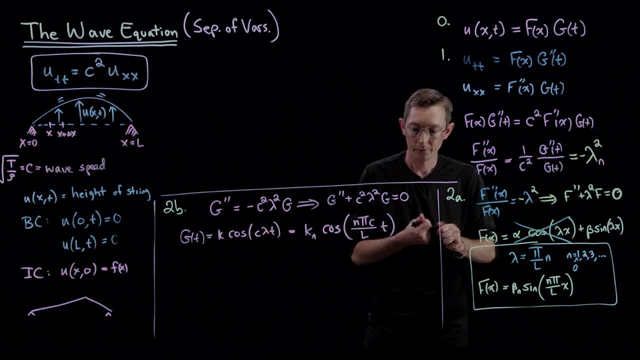 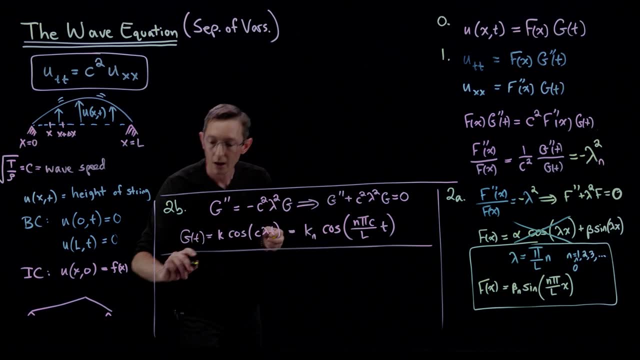 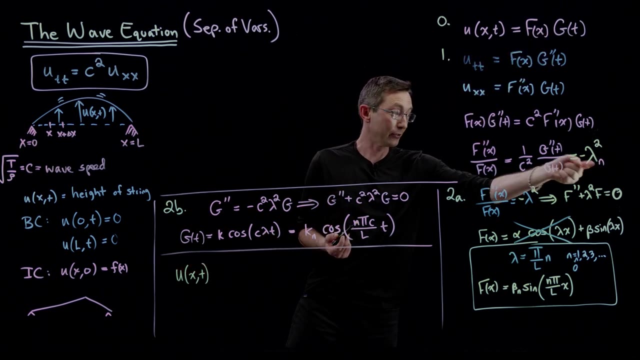 I essentially get my answer, which is: let's see if I can not botch this. it should be pretty simple: U of x and t. remember it's the product of all of these. For every n, for each integer n. 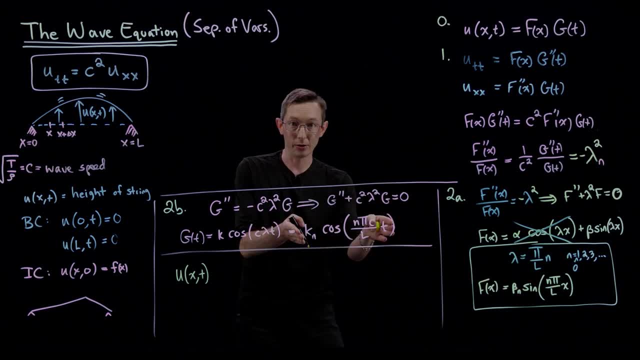 it's the product of this sine and this cosine. And I add up all of those solutions for all n because this is a linear PDE. so all of those solutions are solutions and when you add them up it's still a solution. 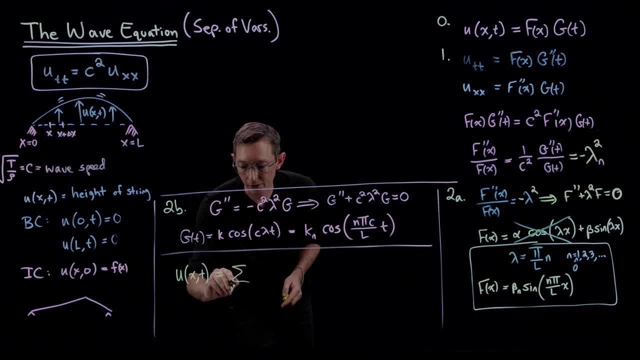 So this is equal to the sum, let's say, from n equals, you know, zero to infinity. and I'm going to just combine these two constants, my beta n and my k n. I'm going to multiply these together, so that's just some constant n. 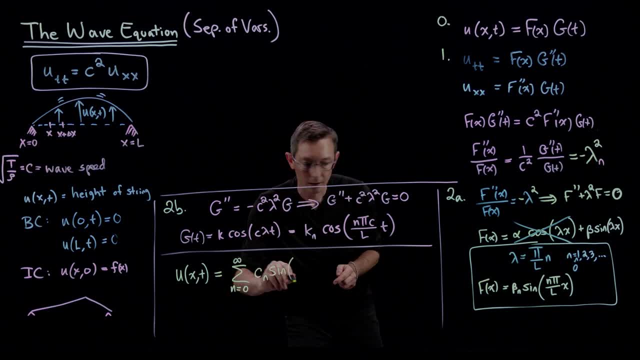 of you know, sine n pi over l x times cosine n pi c over l t, and this is the solution of my wave equation. That was the worst star I've ever drawn, So this is the solution of my wave equation. So u of x and t. 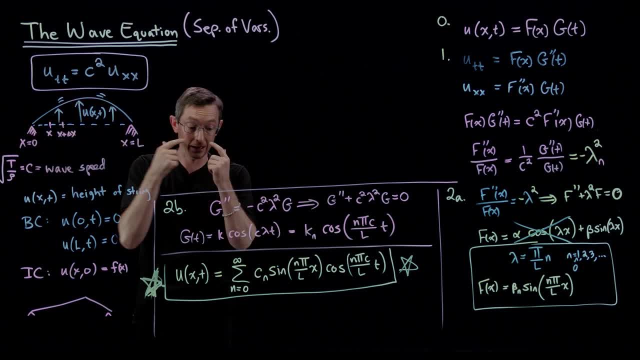 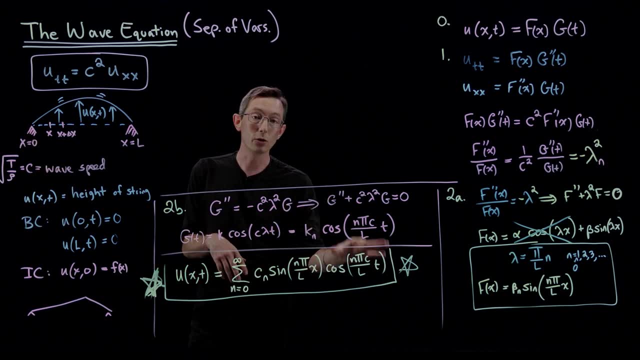 the displacement at every point x and every point time is given by this infinite sum of the products, of sines in x that satisfy my boundary conditions and cosines in time And, if you like, what we're going to do, the way that we determine. 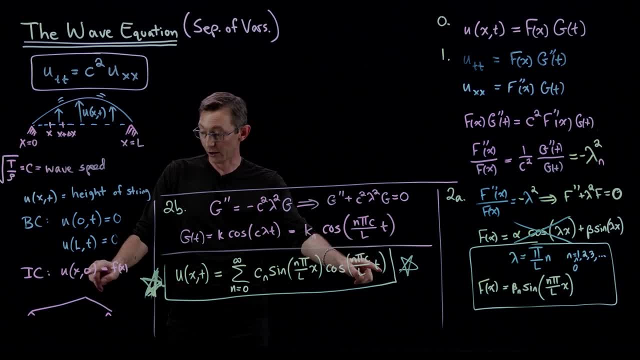 these coefficients is we pin, we use our initial condition, we say: time equals zero, so all these cosines just become one cosine of zero is one, so these go away and we basically say: you know u of x at time zero. 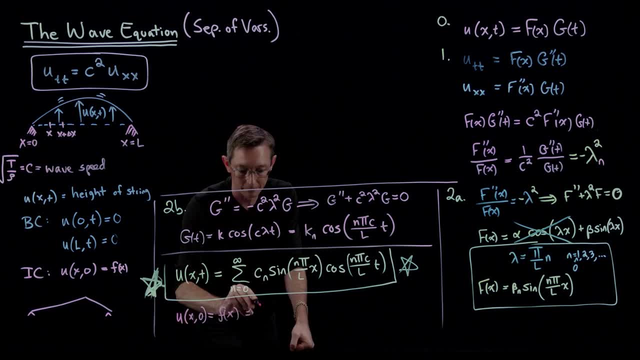 is equal to f of x is equal to the sum of n, equals zero to infinity of c n sine sine n pi over l x, And so that literally means that these c? n's are the Fourier coefficients. if I Fourier transformed my initial condition f, 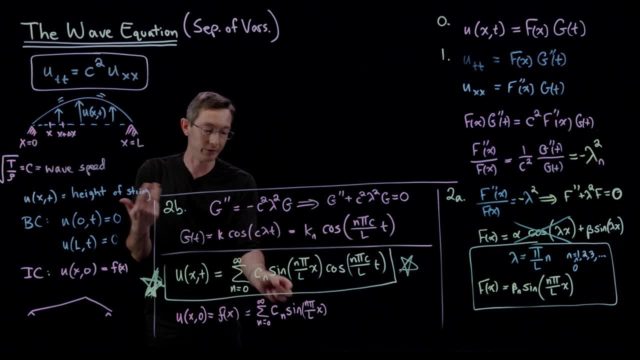 So these c? n's are literally f? hat. They're the Fourier transform, the discrete Fourier transform of this initial condition over that domain zero to l. Okay, And if you, if that was a little fast for you- you can go back to that video. 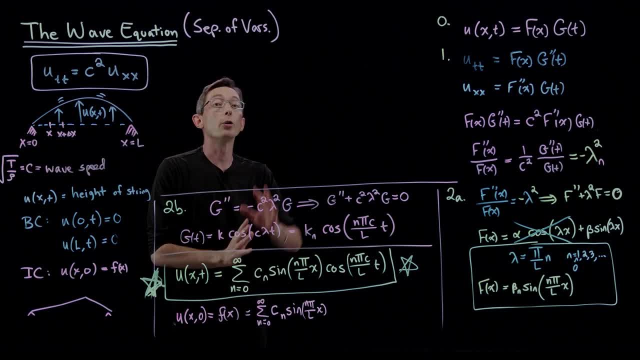 on separation of variables for the heat equation. or you could go to my lecture on the discrete Fourier transform, Like. this is literally the definition of the Fourier transform where these guys here this is literally my f- hat Fourier transform, the Fourier transform of f. 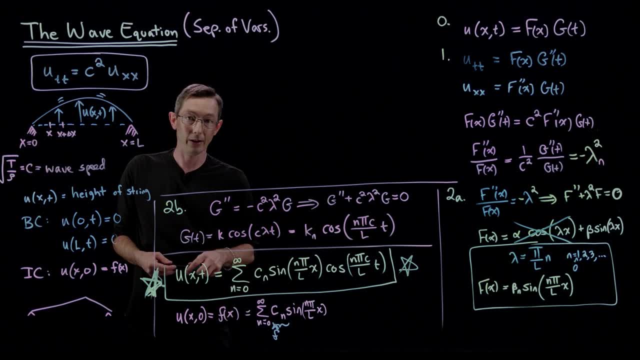 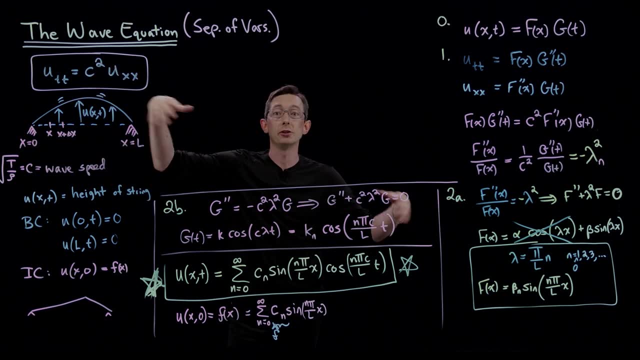 These are my Fourier coefficients of f of x. That's it. That's the whole story. That's how you solve the wave equation: using separation of variables. It's actually pretty easy. It's actually quite simple. You assume that you can split. 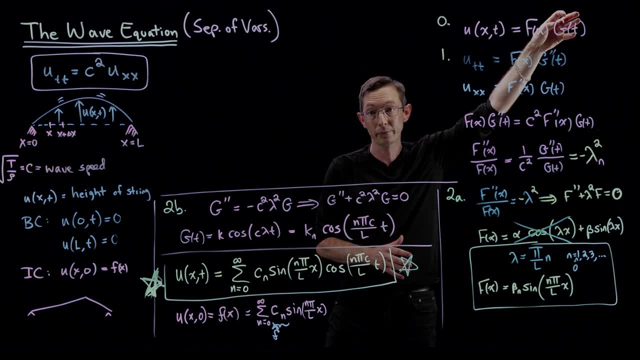 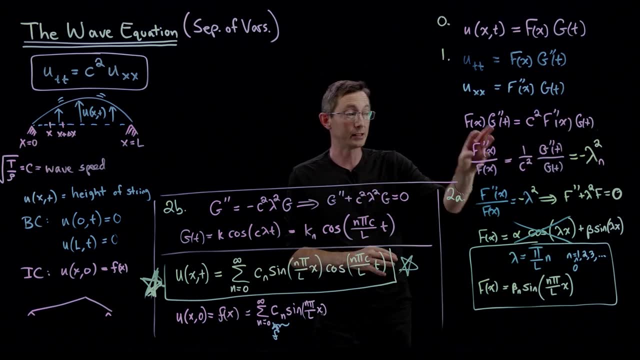 your function into a product of a function of space and a function of time. You plug that into this partial differential equation and take all the derivatives and get you know a relatively simple expression and collect all the terms in x and all the terms in time. 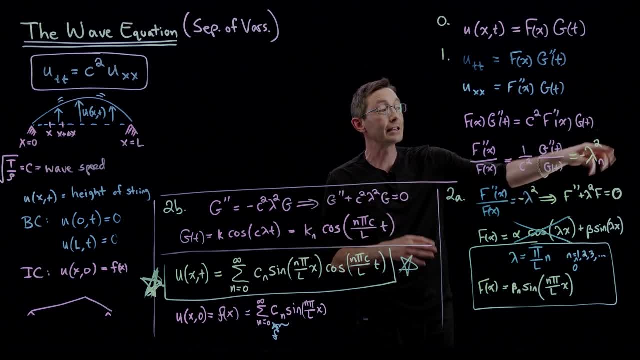 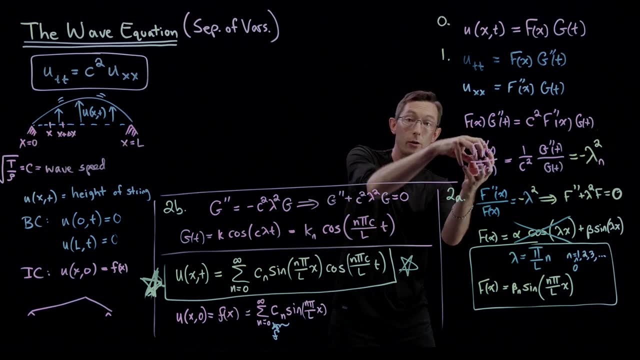 And because those equal each other, they have to equal a constant. And at this point we don't know what this constant is, It's just some constant k. But then what you do is you try to solve this ordinary differential equation for just my spatial variables. 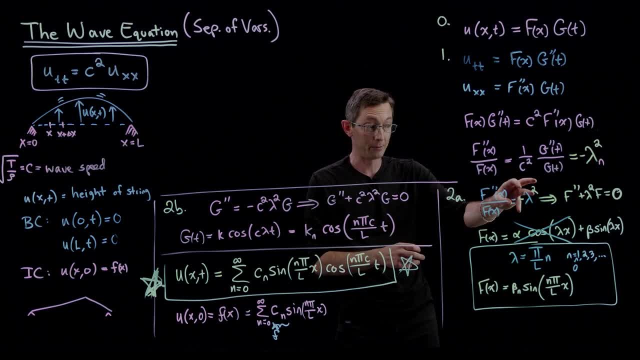 You know, f double prime x over f of x equals some constant, And the only way that that can satisfy my boundary conditions is if this constant is a very, very special number: pi over l times an integer. The only way that we can satisfy 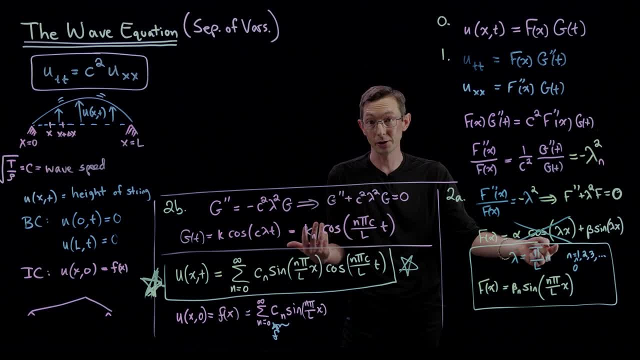 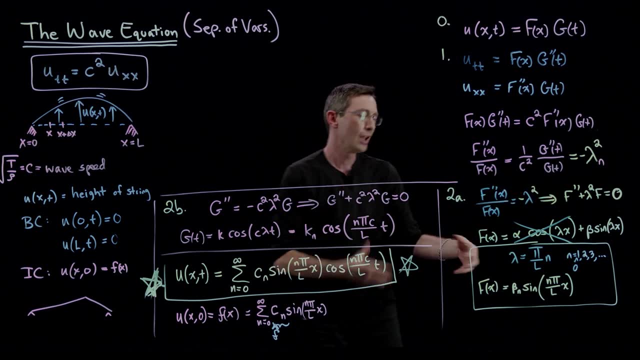 this boundary condition is if lambda is pi over l times an integer. So those are my eigenvalues of this ordinary differential equation or of this partial differential equation. The corresponding eigenfunctions of this are these: sines with that wavenumber, with that lambda wavenumber in x. 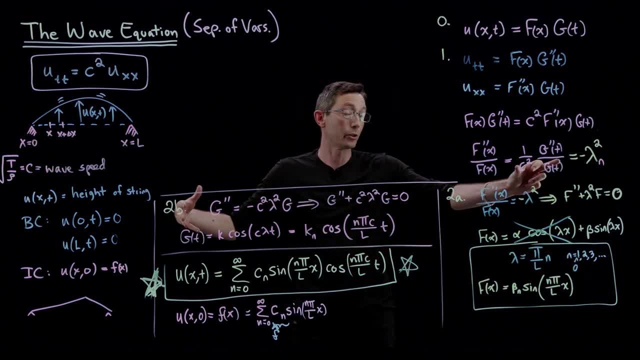 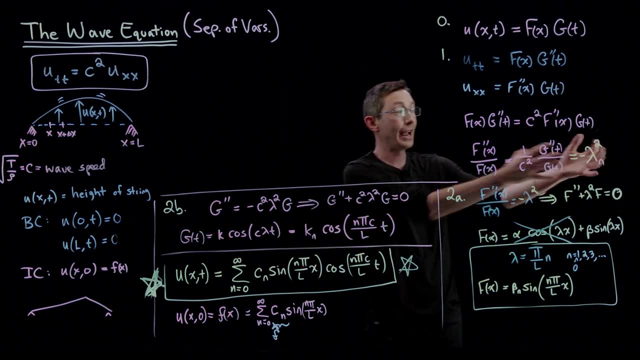 Then you do the same thing for my ordinary differential equation in time. Now that I have determined what that eigenvalue lambda has to be to satisfy my boundary conditions, I have to use that same one for my ordinary differential equation in time. So now I get these sines and cosines in time. 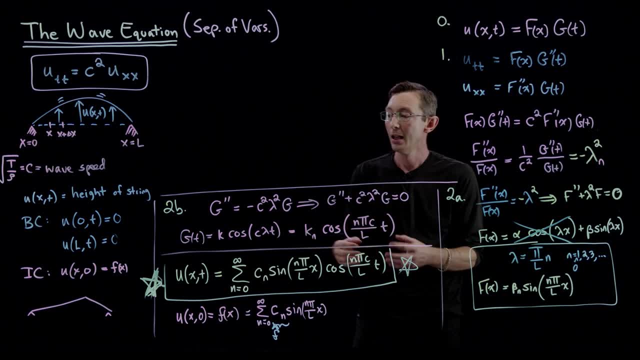 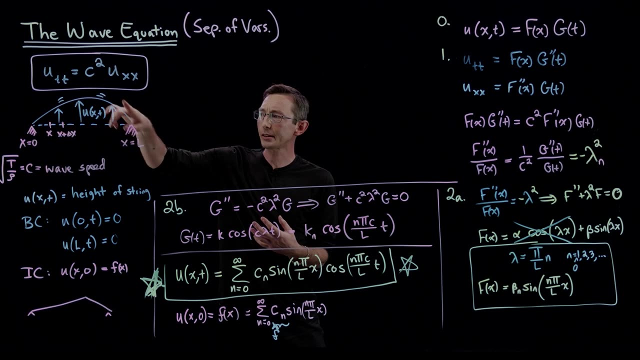 with a slightly different frequency, And when I combine those two solutions, when I take their product here and I add them up for all integers n, I get the solution of my partial differential equation. And what that means physically is that the solution of this partial differential equation. 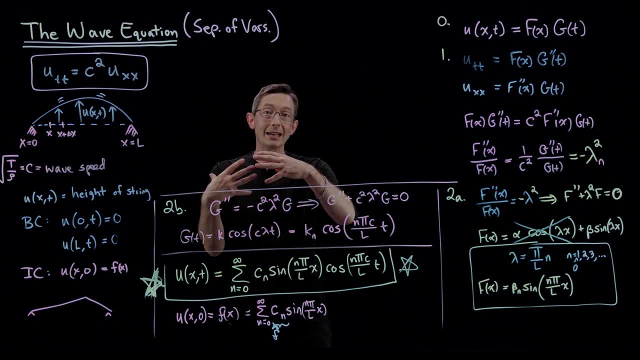 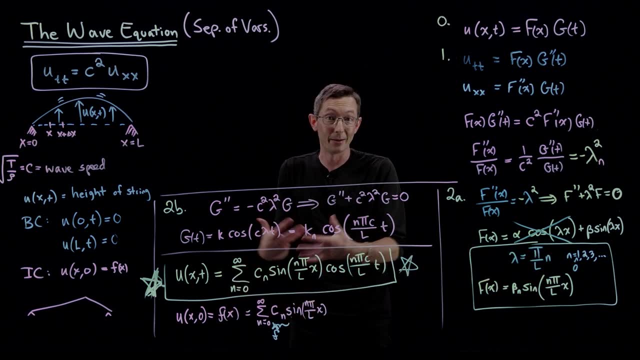 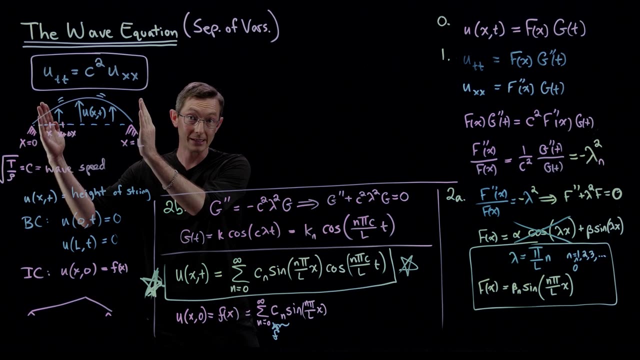 I basically take my initial condition and I, you know, decompose it into a bunch of sines. I take its Fourier transform to find out how I can add up infinitely many sines with, you know, period l. you know all of my sines with period l. 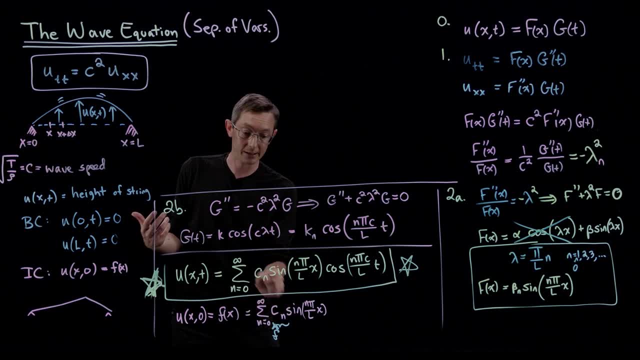 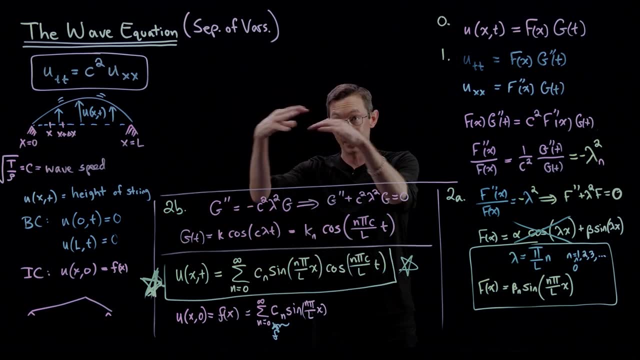 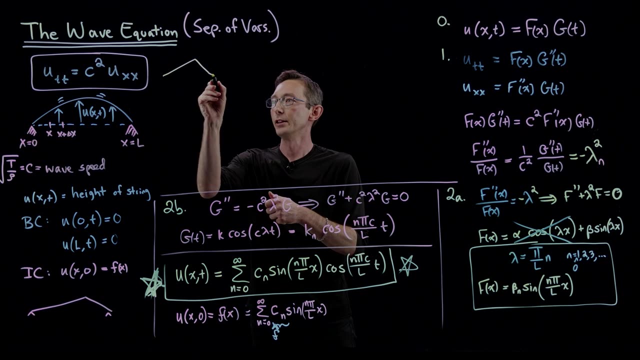 And that determines this constant c for my solution. And so then, each of those independent kind of harmonic components, each of those independent sine waves, we're literally saying, you know, if I have some initial condition, like maybe what I do is I pull up the guitar strings, 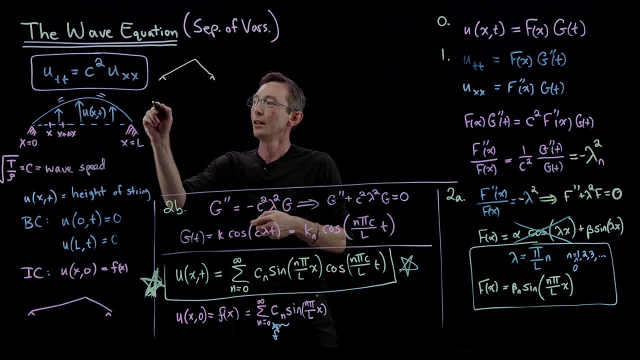 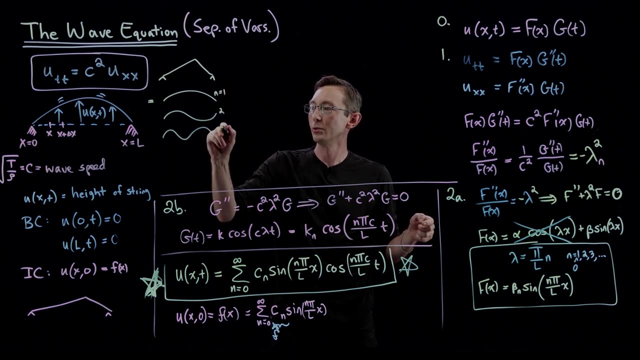 with my finger and I make this little triangle that is equal to the sum. of you know, this sine wave plus this sine wave, plus this sine wave, and so on and so forth. This is the n equals. you know one, two, three, four. 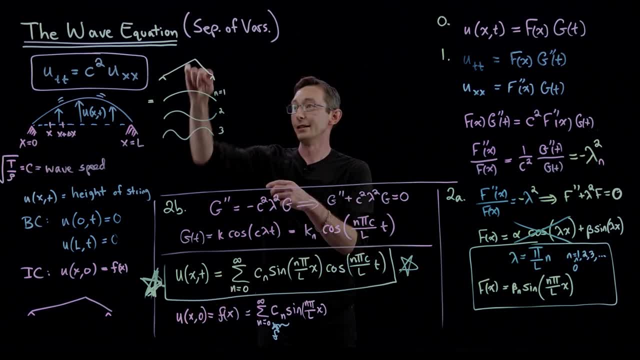 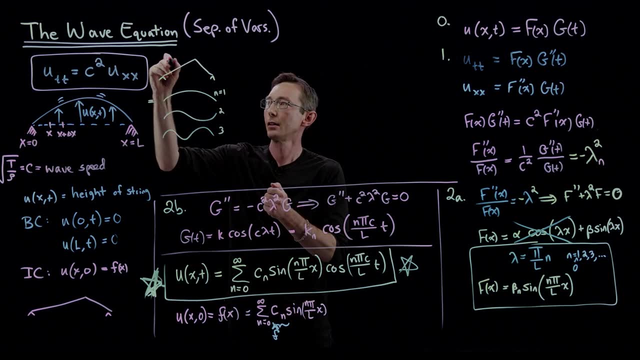 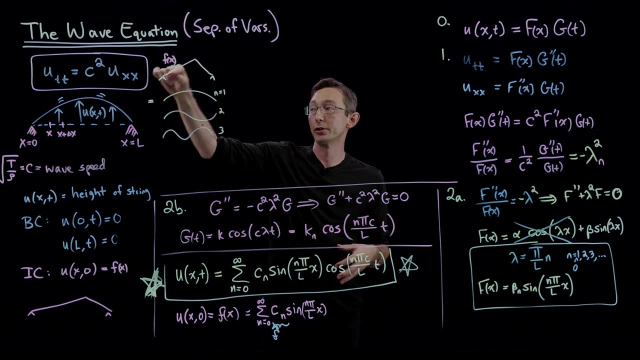 and so on and so forth. And you know, the coefficients cn are given by the Fourier transform of my initial condition. This is f of x. Then each of these components, these wave components of my initial condition, oscillate at a different frequency. 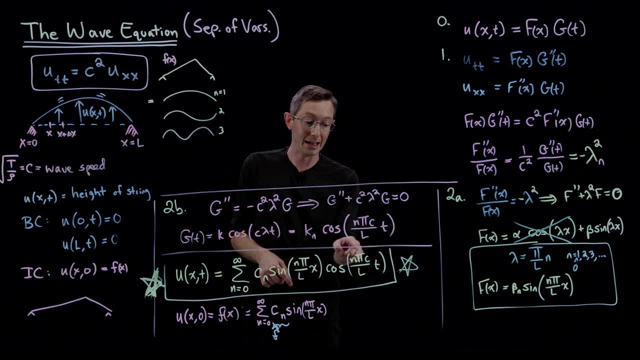 So this n equals one component, oscillates at a frequency n, pi c over l, The n equals two oscillates at twice the frequency, n equals three at three times the frequency, and so on and so forth, And so essentially you know, 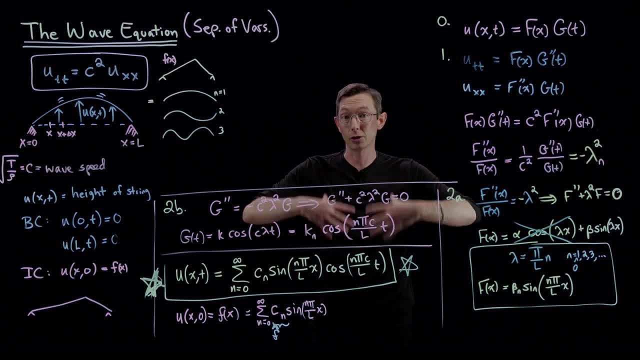 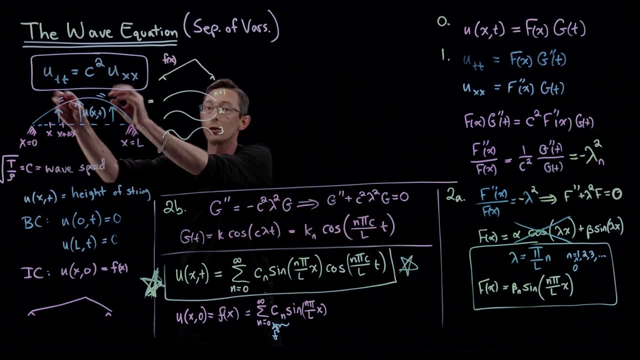 this vibrating guitar string is causing pressure fluctuations in the air that it's sitting inside of and that's what's creating the acoustic waves that are radiating away from this that you can hear when someone plays the guitar or when someone plays the piano. Okay, it comes from literally. 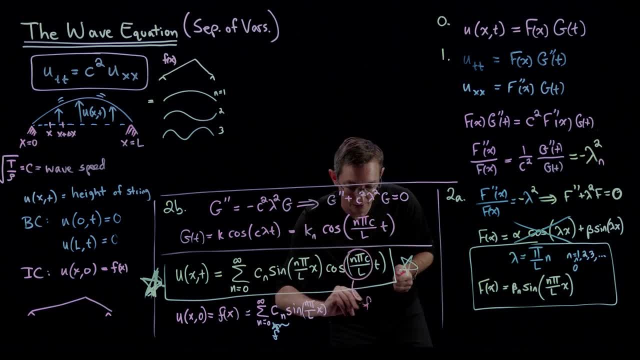 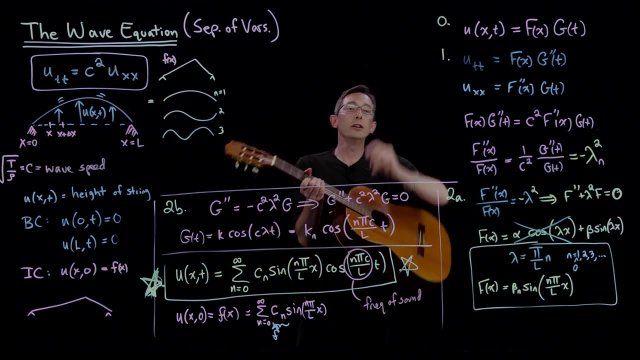 from this frequency here. This is going to be the frequency of sound that you hear. is this n pi c over l? And so now we actually see very clearly- and I'll pull out the guitar again- for this is: we knew that the wave speed depended on things. 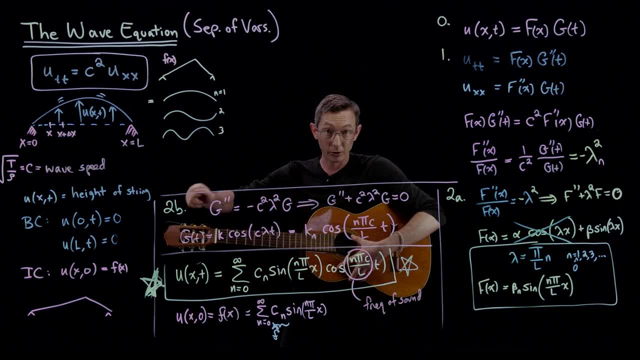 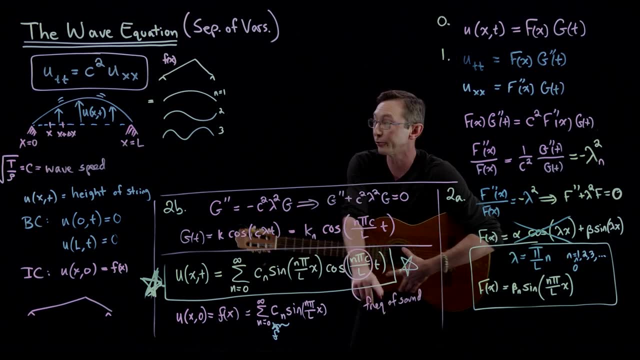 like the tension in the string. So you know, if I increase the tension it should increase the speed. And so now we know directly that increasing the tension will increase the frequency of acoustic waves, because this is the oscillation in time that's creating those acoustic waves. 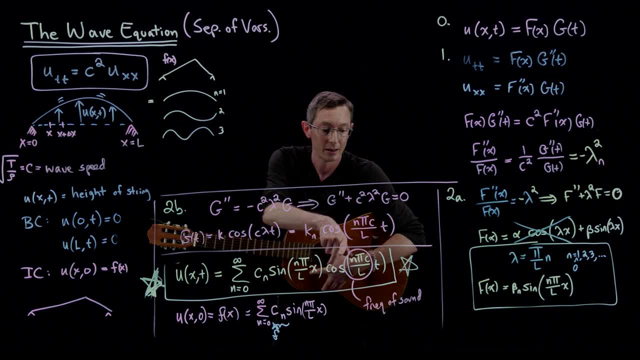 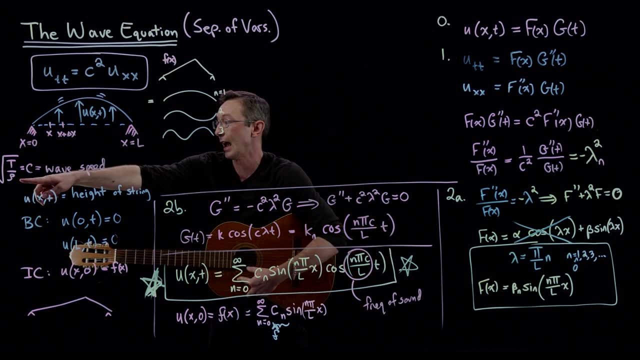 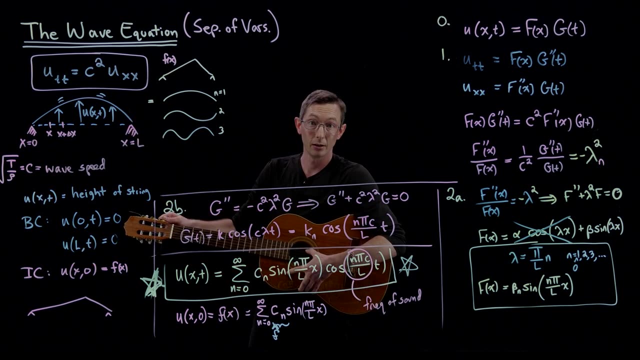 Kind of how fast this thing is flapping in time is n, pi, c over l. So increasing c, like increasing c by having a smaller string, makes a higher-pitched sound. Increasing c by increasing the tension also increases the sound. But the other thing that could you know. 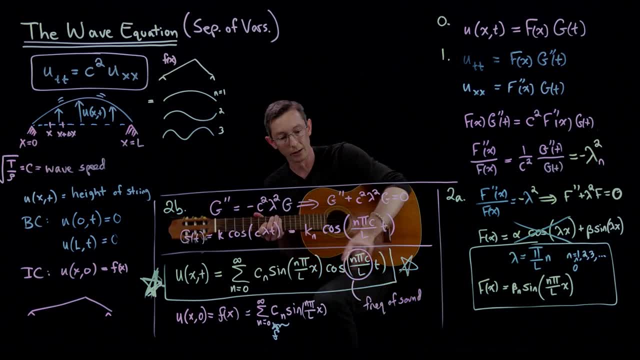 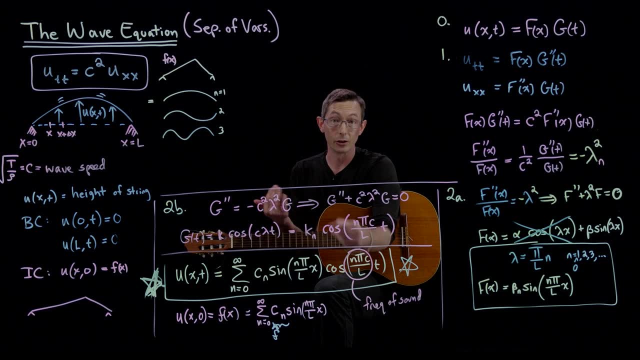 increase the frequency, the pitch of the sound you hear is changing l. So if I make l smaller, if I cut l in half, this frequency should double. So if I take my length and I pick the middle point of the length, 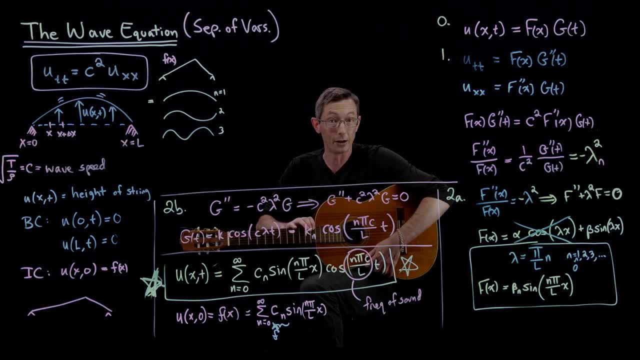 I think you can see this: the middle point here. this is the 12th fret. the middle point is twice the frequency. Okay, so changing l, you know, if I cut l in half, if I pin this thing, so it's half the length. 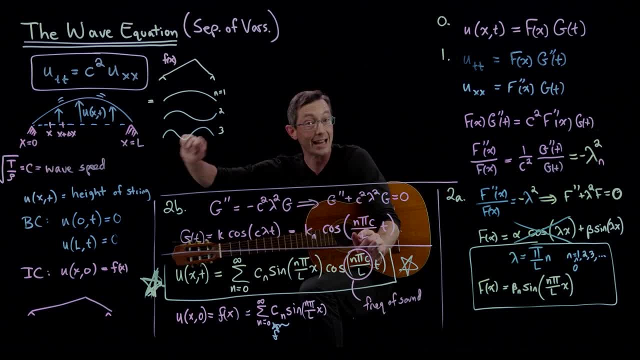 it's going to be twice the frequency. Or I could increase the tension by a factor of, I guess in this case 4.. If I made 4 times the tension in the string, it would double the frequency. Or if I made it 4 times less dense. 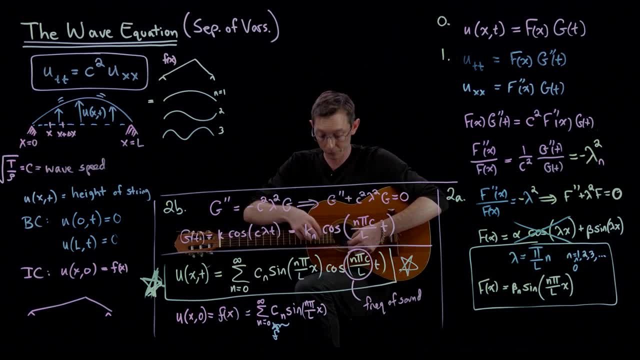 if I ever picked a material that was 4 times less dense, or I made it 4 times smaller, those would all have the same effect of changing the frequency of the sound. Something else I think is kind of neat is if you picture, you know. 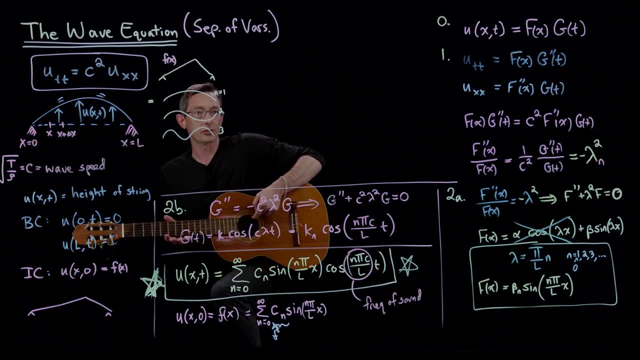 I'm literally like pulling this guitar string up, so it's a little bit, you know, like a very, very shallow triangle when I pull it up, And that's my initial condition, and then I let it go. You can picture the sum of all of these waves. 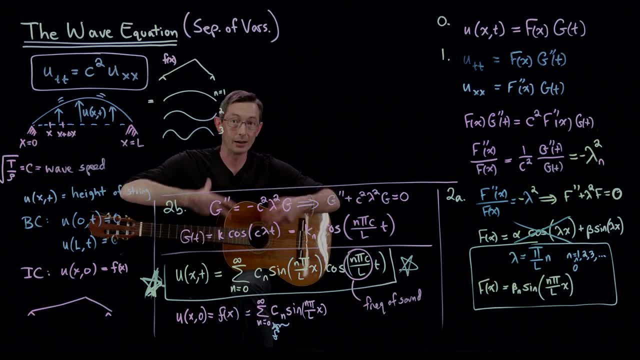 oscillating in time kind of the amplitudes are oscillating in time to generate that sound. And so if I just very lightly hold down the string at just a random location, you hear that it's really damped. You don't hear anything that sounds. 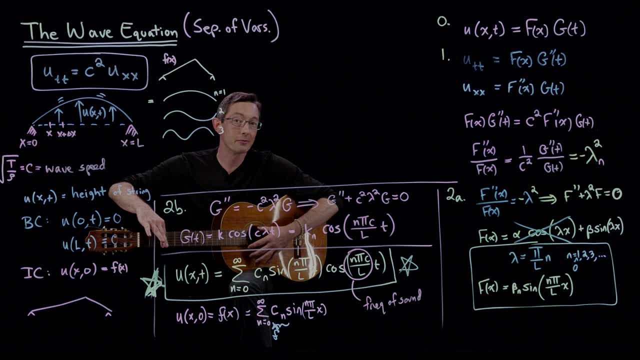 nice, like a chord, It just sounds damped. But there are some very special locations where some sound does come through. Here's one, And I believe this is a third harmonic. It's a third of the length of the string. So you know some of these waves. 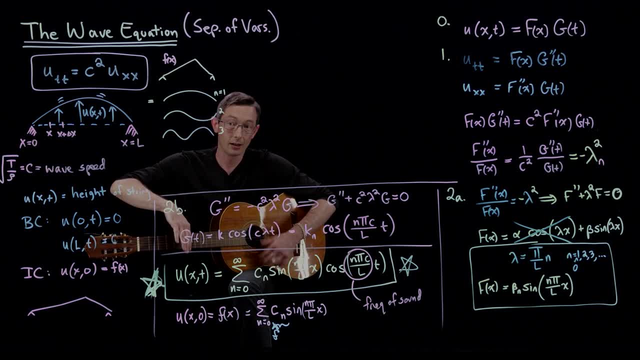 have a node, a zero point at that location And so they are not affected by me damping at that location. And you can hear this really, really clearly. If I move my finger very lightly on the 12th fret, you can see that most of the sound. 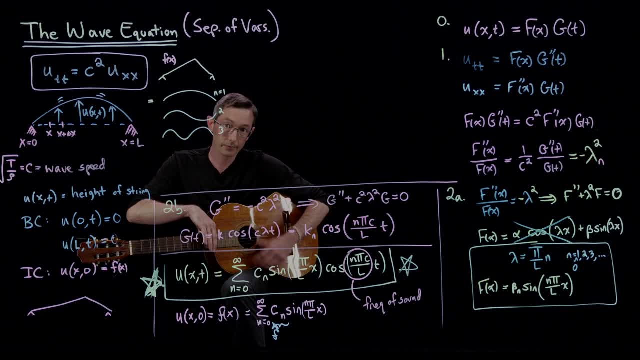 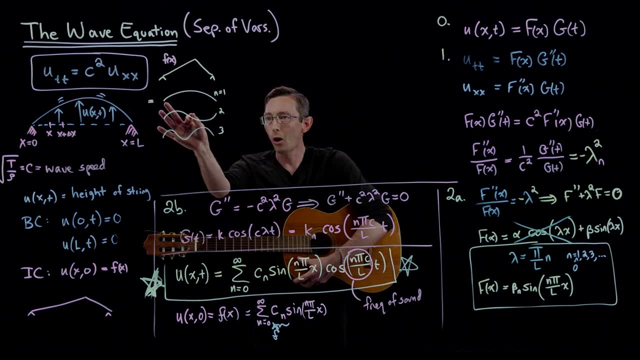 is coming through And it's a little bit higher pitched. That's because all of the even ends- n equals two, n equals four, n equals six- all of those even ends are being able to come through, Even though I'm damping. 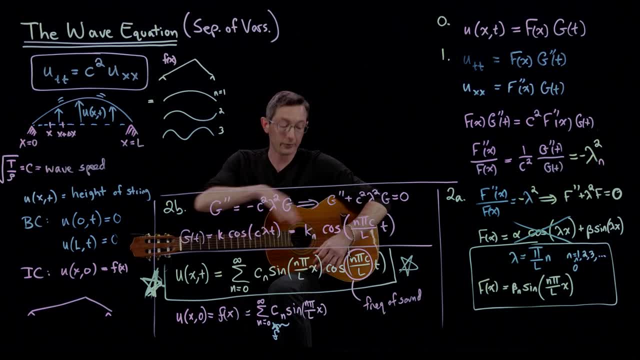 I'm kind of like holding a little bit of a damper at this point. All of the even end sine waves are not affected, because they perfectly kind of pass through that zero point where I'm holding my finger, Whereas if I pick a random location, 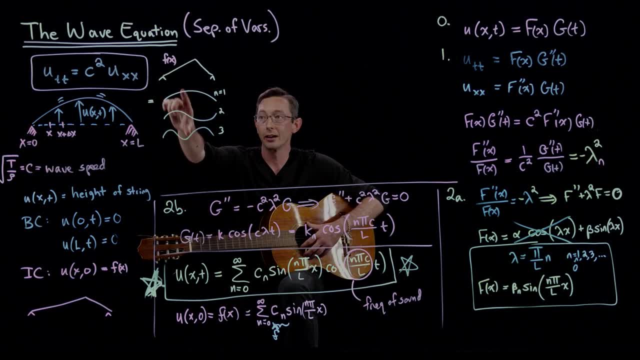 and I put my finger there, I'm kind of killing all of the waves and I'm killing all of that sound. Maybe this will make more sense if I pick one string And it's twice. the frequency n equals two, So that's kind of cool. 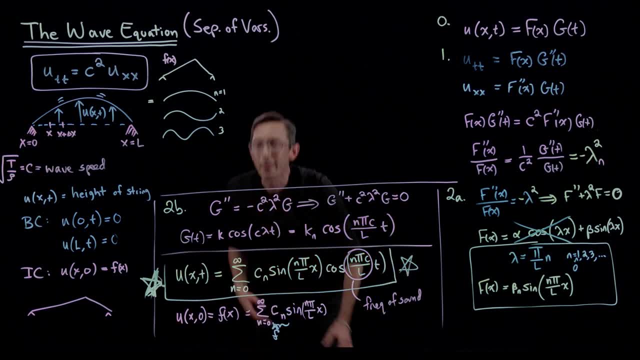 Anyway, this is just an example of how you can get some intuition. So I always like to think about these kind of wave physics. with an intuitive example, You could pick Maxwell's equation. You could pick, you know, ripples on a lake. 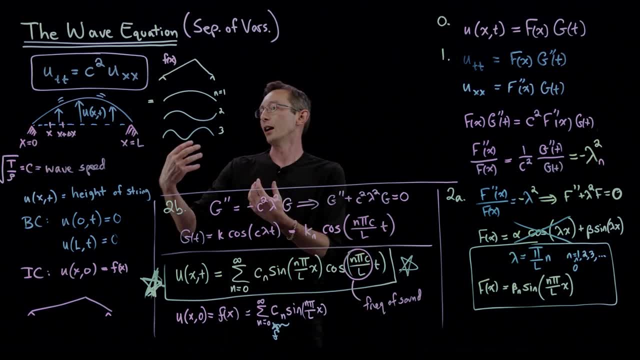 I like the guitar string because I think it's very intuitive how these sounds are being generated. You can put your finger in different places. You can put your finger in different places to change l. You can increase the tension or decrease the tension. You can go to a string that has lower density. 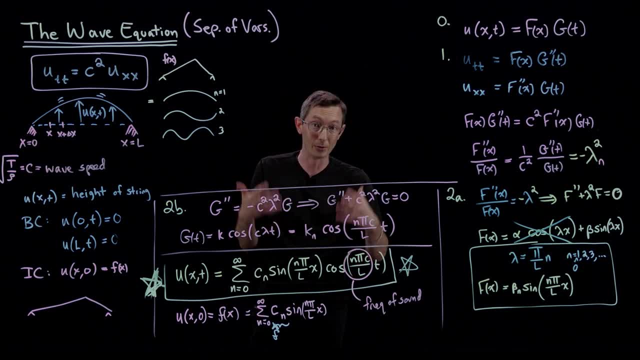 or higher density, and all of those change the frequency of the sound. Good Yeah, one last thing I want to show you, and this is going to end up being an entire additional lecture, So I'm going to very likely have a whole lecture. 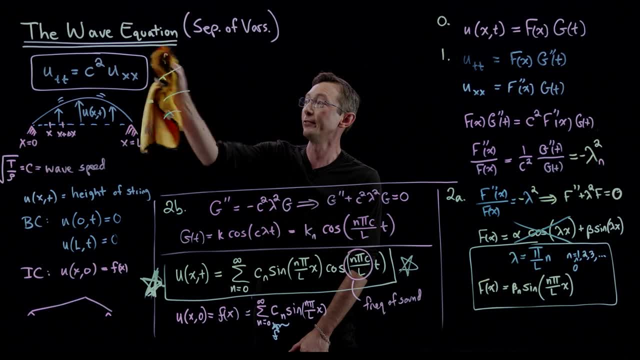 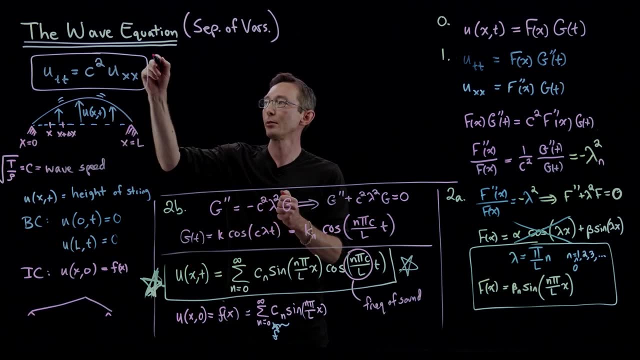 on the method of characteristics, which is a very, very, very important idea. in these. This is called a hyperbolic. This is a hyperbolic partial differential equation. So this is a hyperbolic, hyperbolic PDE. 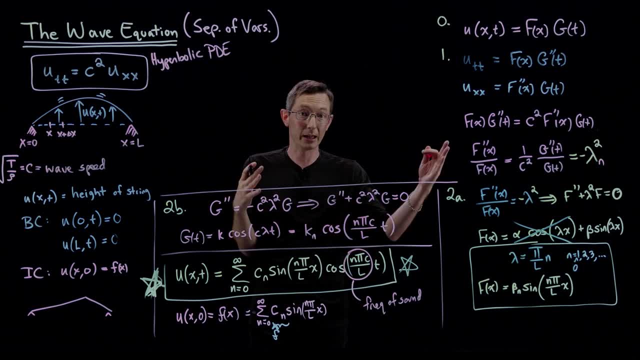 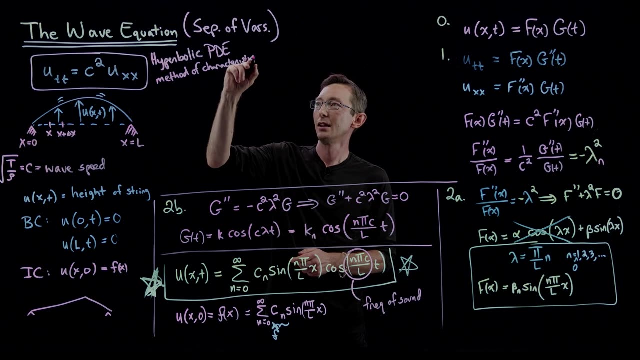 which basically means that there is a speed of information propagation in the problem, because there's a speed of sound, And for hyperbolic PDEs there is something called the method of characteristics. Method of characteristics. I believe this was also invented by d'Alembert. 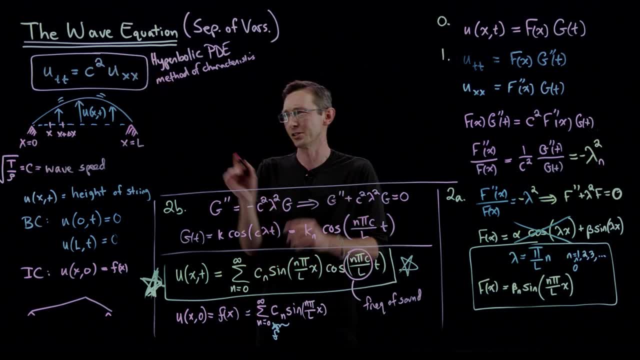 when he derived this wave equation. I'm not 100% sure, but I think so, And I'm going to have a whole lecture on this. But what I want to show you is that when you have sine of something times cosine of something. 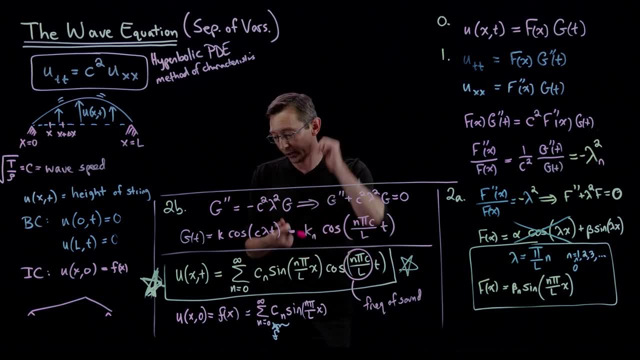 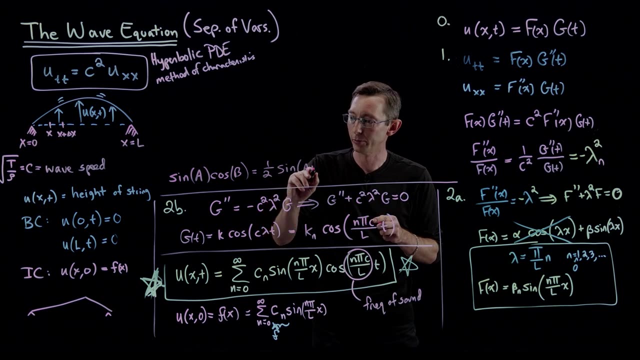 you can use the trig identity, a really really simple trig identity, which is sine of A times cos of B equals one half sine of A plus B, plus sine of A minus B. This is just a trigonometric identity. You can verify this yourself. 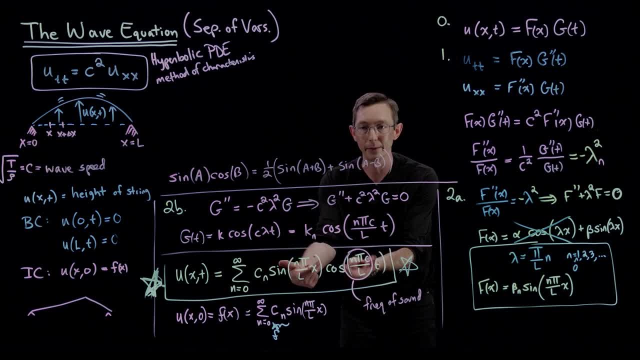 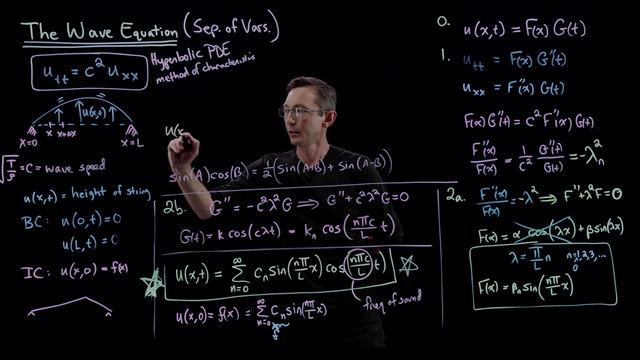 But because all of our solutions have the form sine of something times cosine of something, I can essentially use those to write down the following. Essentially, my solution is going to be: you know, u of x and t equals. I don't want to write this. 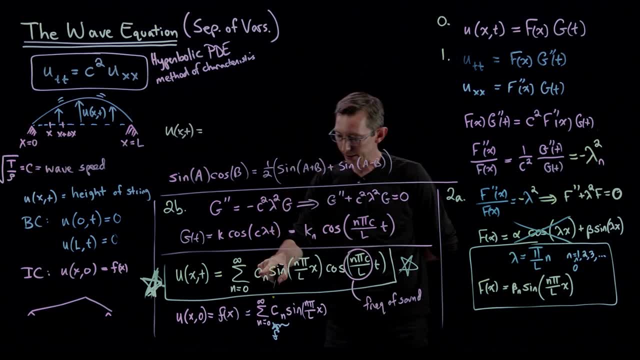 I'm going to say this is equal to the sum from n, equals 0, to infinity of that constant cn divided by 2 times. now I'm going to have sine of this plus this, plus sine of this minus this, So that's sine of. 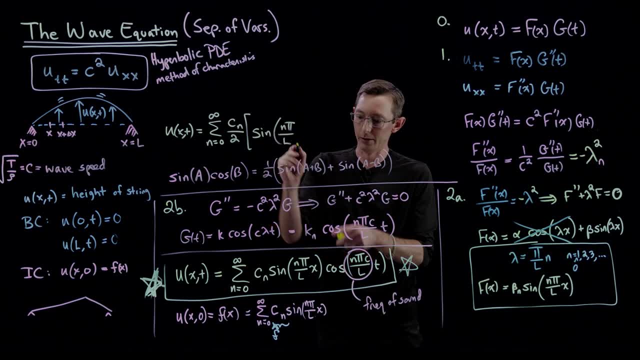 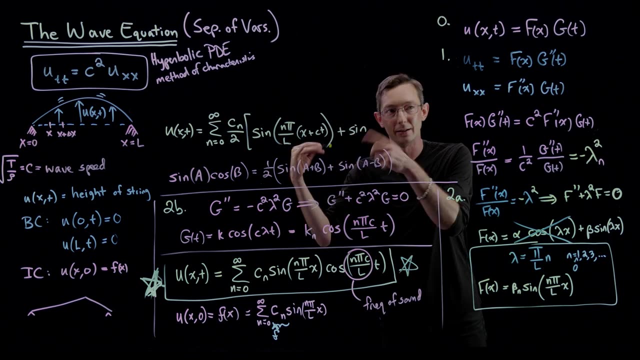 n pi over L x, plus n pi over L ct. So I'm just going to say plus ct And plus sine. I'll go back and we'll double check that I didn't mess anything up: n pi over L. and now it's this minus this. 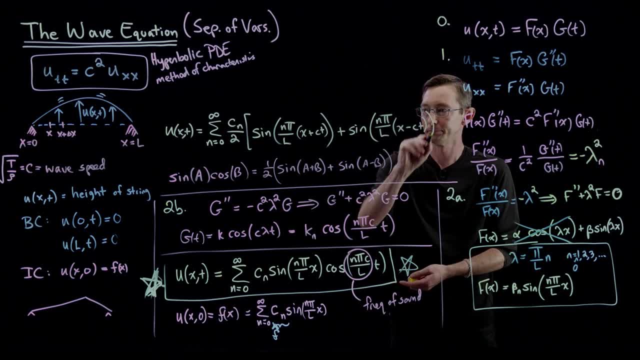 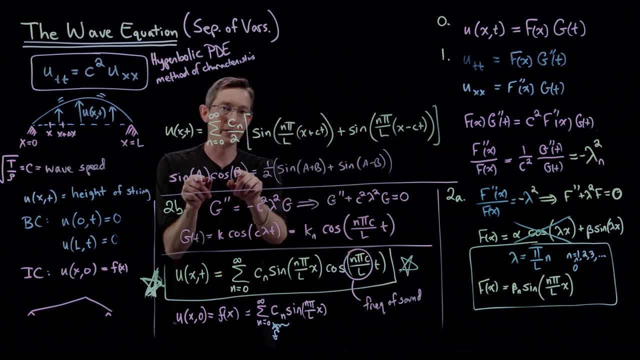 So that's x minus ct, And so this is really really, really interesting. What this says is that, because of this trig identity, sine of a times cos b equals, you know, one half sine a plus b, plus sine of a minus b. 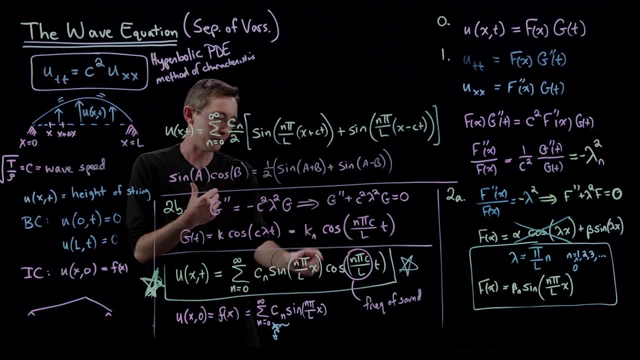 I can take these and you can verify for yourself that you know n? pi over L times x and n? pi over L times ct. give you this expression. when you use this trig identity. What we find is that essentially our solution u of x and t. 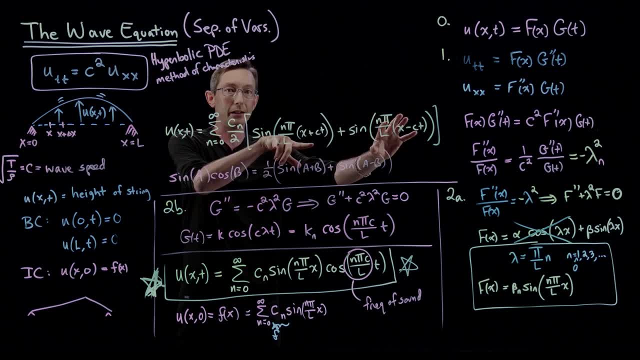 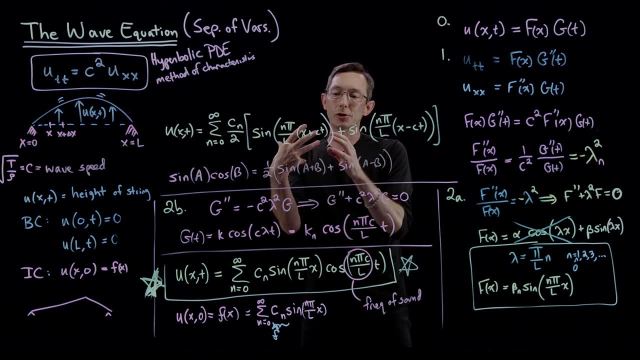 is given by two. these are called waves that are traveling in different directions. So x plus ct is a solution that is traveling in one direction. As time increases, this is kind of shifting my solutions. I think this is shifting my solutions if time increases. 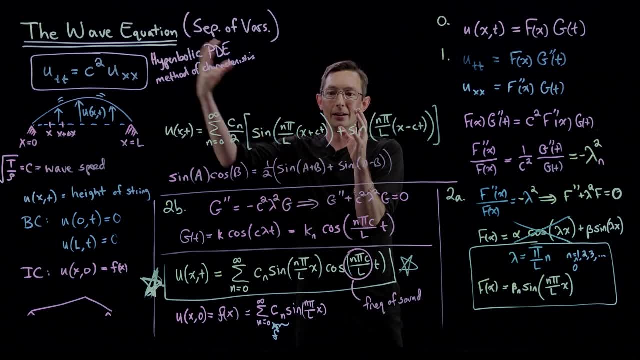 then x has to be positive, x has to be, you know, negative to make this zero. And this other part here is traveling in the other direction. So I'm just going to draw a little picture here. This is like a teaser for later.